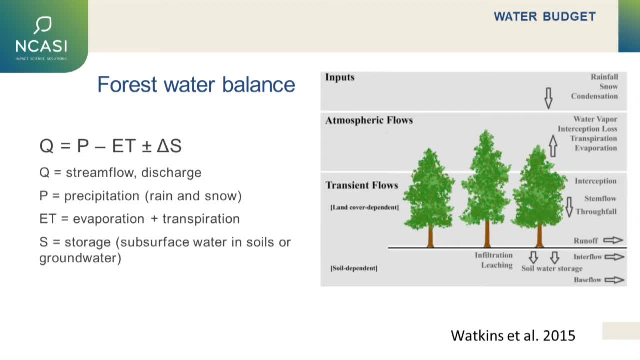 is really the function of changes in your inputs and outputs. Inputs, of course, include precipitation, as rain, snow, also condensation, such as fog. but our outputs can include transpiration from trees but also evaporation from the entire ecosystem, And so evaporation is from all surfaces in the ecosystem. 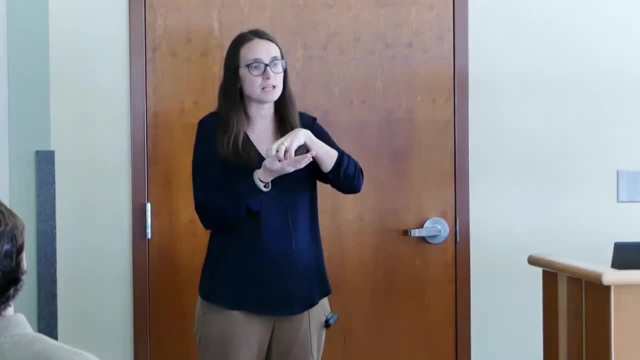 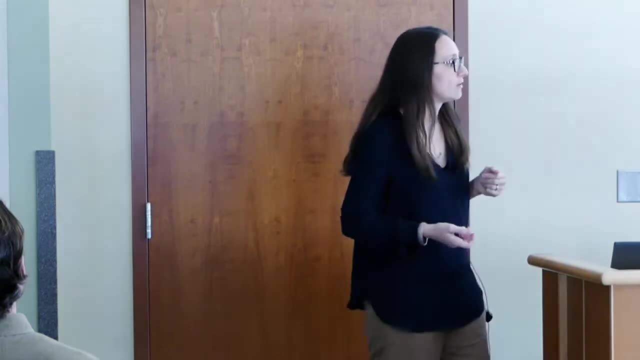 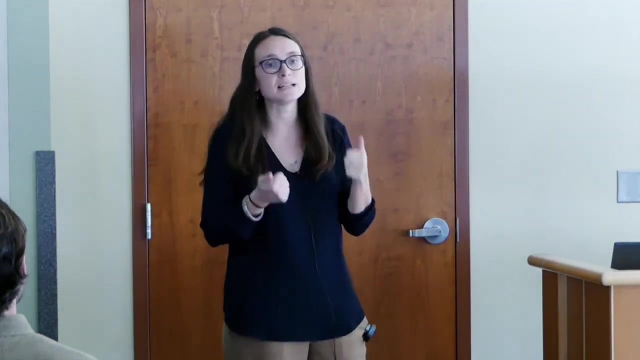 so that includes water stored that's intercepted by tree canopies, that can evaporate to the atmosphere as well as, on the forest floor, evaporation from those surfaces as well. And then the other component, which can be a plus or a minus depending on the system, is subsurface storage. 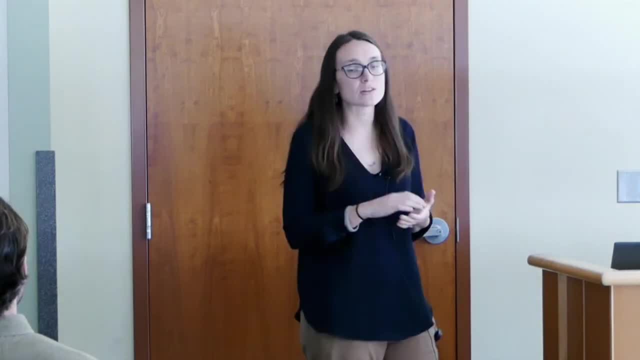 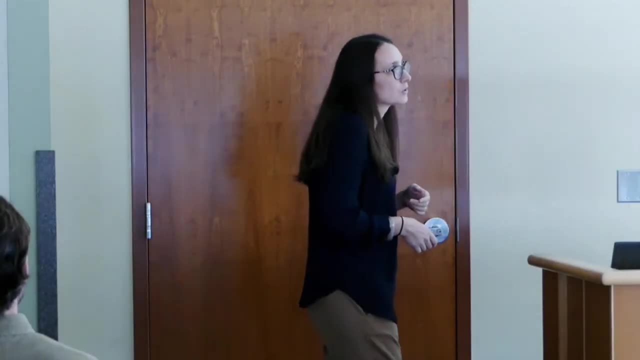 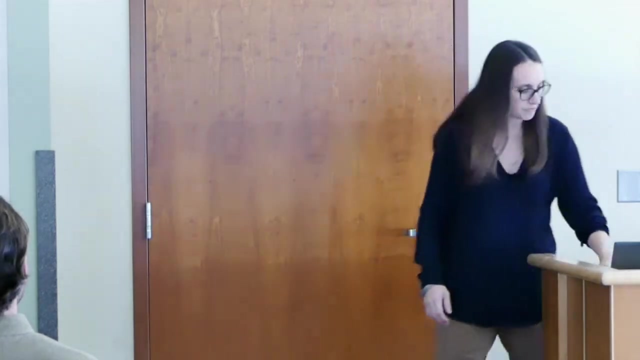 So storage components for water include water that's stored in soils, so in upper layers of soils, but also in deeper groundwater locations. So base flow is a function of those storage components, And so at a typical hydrograph our base flow basically refers to: 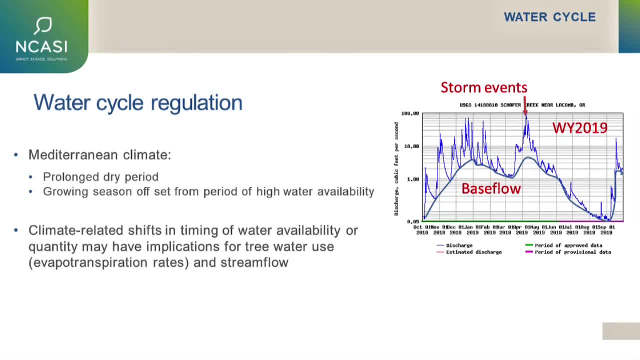 our base flow basically refers to flow that's supplied from groundwater sources to the stream in between storm events, And so if you look at this hydrograph, you can see the spiky nature of storm events, in terms of when those precipitation events occur. 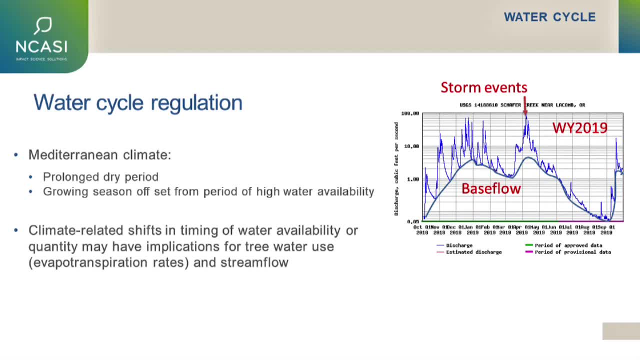 relative to how base flow is changing throughout the year. Here in the Pacific Northwest, we need to talk about the Mediterranean climate that's experienced here. So that means that there's high water availability during a portion of the year and then there's a dry season, which you can see in late summer. 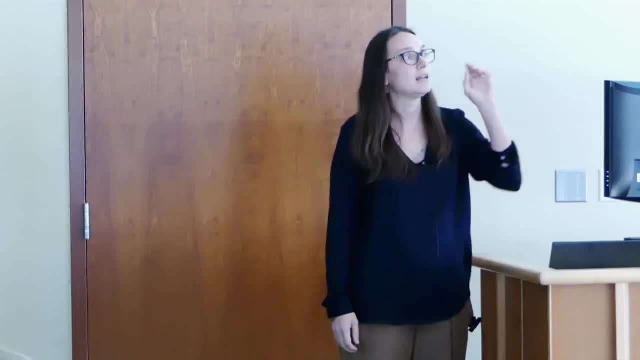 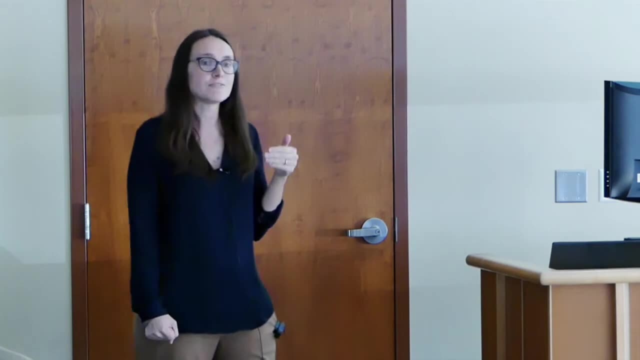 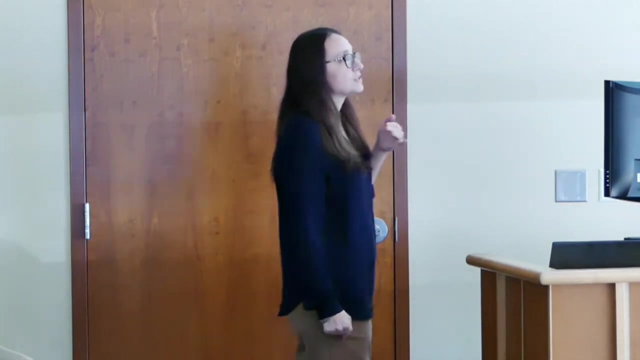 when you see the decline in the base flow condition, And it's important to talk about that because, in terms of tree water relations, the growing season is offset from that season of high water availability And that has important implications for stream flow. So today I'm going to talk a little bit about climate responses over time, 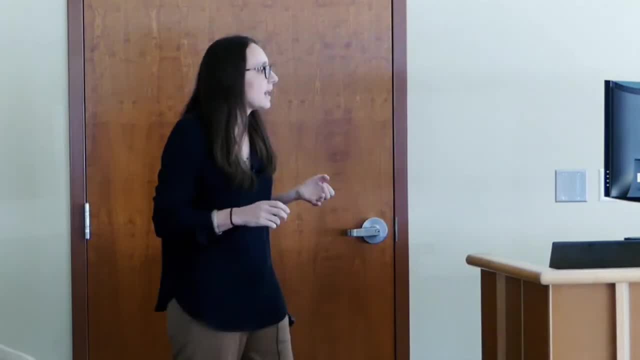 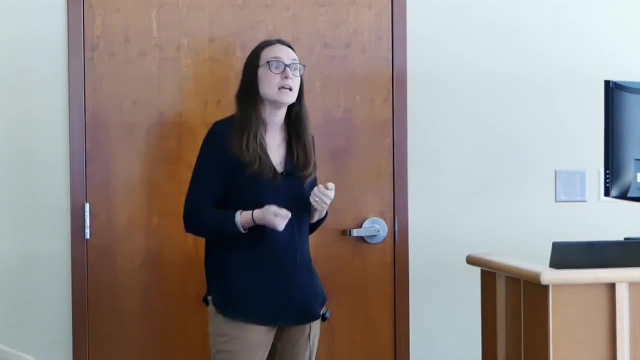 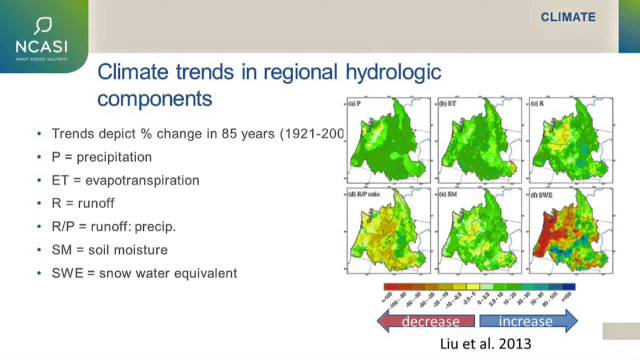 which we already heard a great deal about, and and how those climate related shifts in timing- not only quantity, but also timing- may have important implications for water availability in stream flow annually as well as seasonally. So I'm going to talk about some of those projections for climate trends. 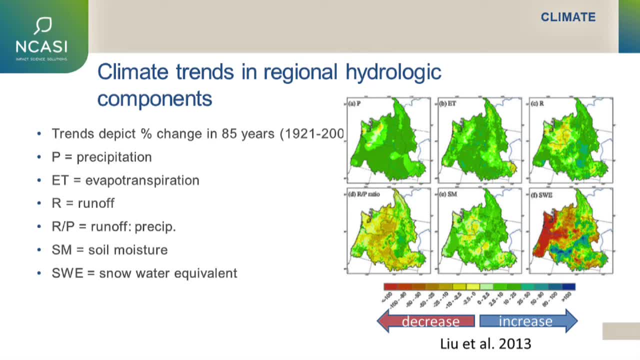 for each of these water budget components. This is one example of all of those components, but I'm going to talk about some more specific examples. So, starting with the component of storage, So starting with the component of storage, So starting with the component of storage, 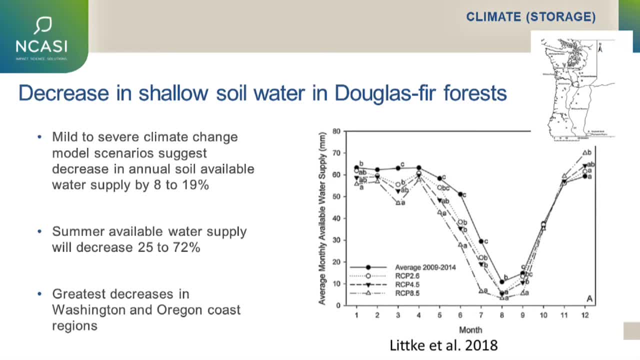 So, in terms of how we expect some of these storage- the storage of shallow soil, water availability- to change with some of these climate change scenarios, Kim Litke and her co-authors from the University of Washington instrumented upper soil layers across Oregon. 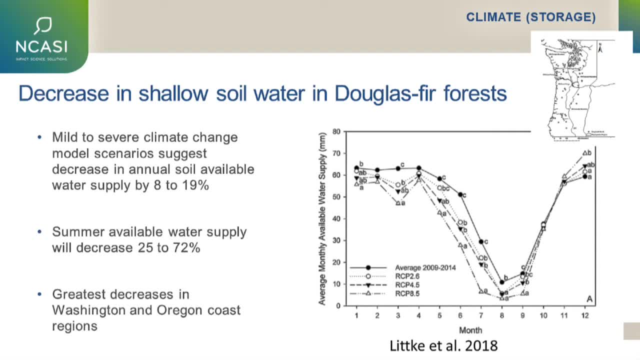 Western Oregon and Washington in Douglas fir soils. And then they used all of that information to to apply to these climate various climate scenarios. They had a moderate scenario, a mild, a mild, a moderate and a severe climate change scenario. 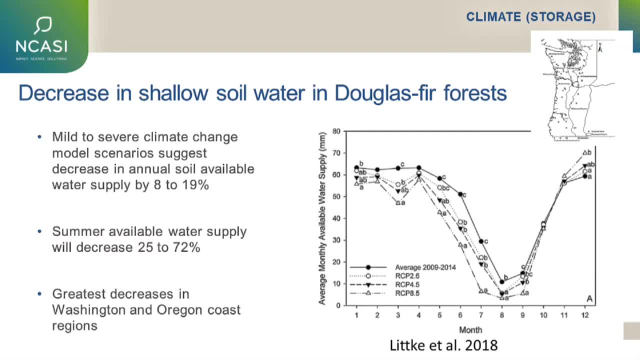 They found that, overall, there was an eight to 19% decline in annual shallow soil available water supply, As seasonally, in terms of summer, they found a decrease in 25 to 72% overall, And they within the scope of their study. 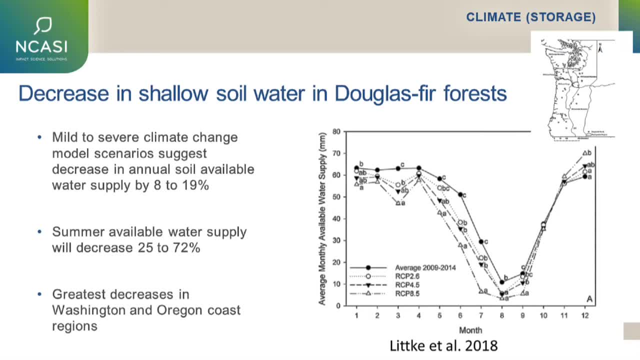 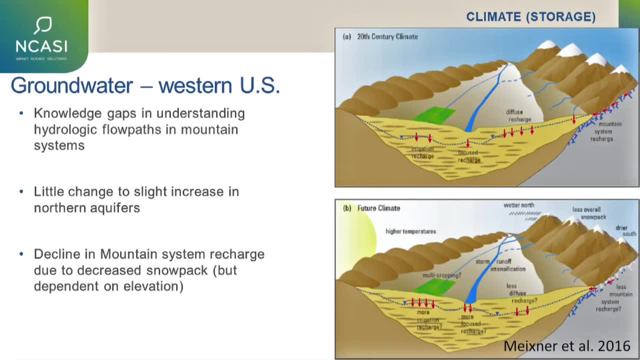 they found, the greatest decreases occurred in coastal regions of both Washington and Oregon. Another component of storage, of course, our deeper groundwater groundwater sources. I would say there's a lot less known about, about this particular component of the water budget. 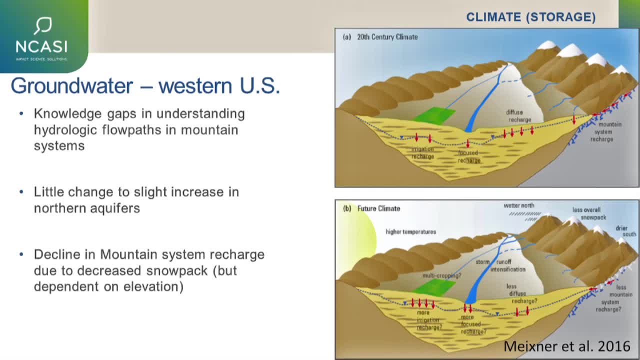 One study. this is a study from Mixer and others in 2016,. they evaluated aquifers for the entire Western us, And so they identified that there are there are knowledge gaps in the. in this diagram, the upper panel is is: is it? 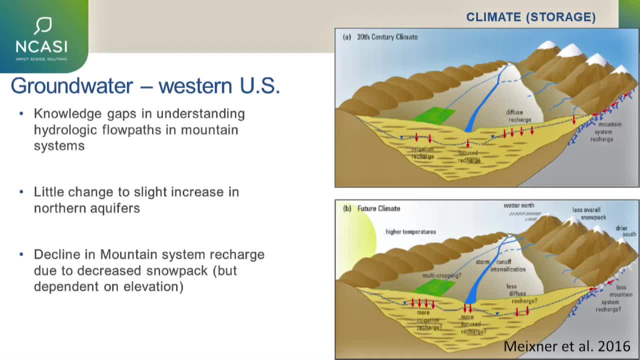 essentially the sort of what those groundwater recharge sources are for the current climate. and then they have another scenario about some of that uncertainty and what that might look like in a future climate. so what they found was that overall there was little change to even a positive increase in. 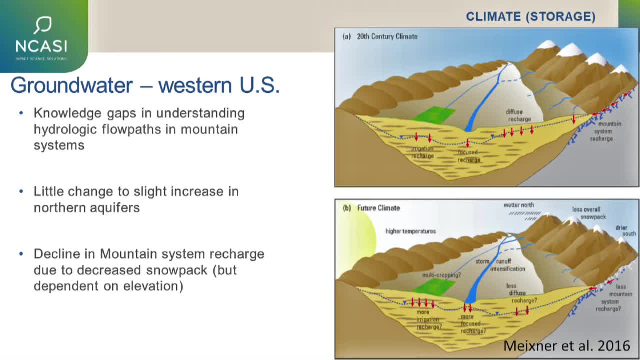 terms of northern aquifer water storage, but they did see a decline in mountain system recharge due to decreased snowpack, but they note that that is dependent on elevation. so so this is informative, but- but this is a certainly an area where there are some major knowledge gaps in terms of what 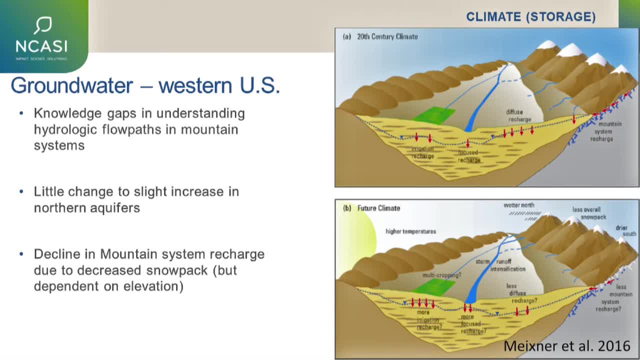 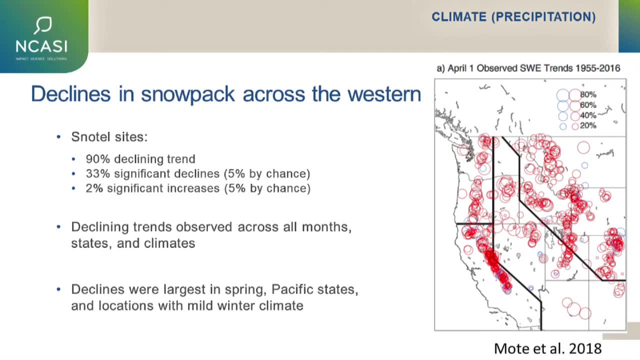 groundwater recharge looks like with climate change. so, moving into the precipitation component, as we heard earlier, one of the major changes in terms of precipitation is the change in snowpack, and that's really. that's really because models are better able to make projections. so that's really because models are better able to make projections. 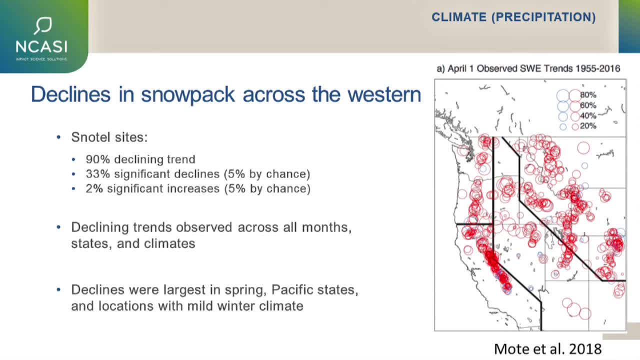 for temperature changes, and temperature change can shift the type of precipitation that's received, so in milder climates there are expected to be more of a decline in snowpack. this paper is moat and others updated their 2005 paper with a more recent analysis across all the snow tell sites in the western. 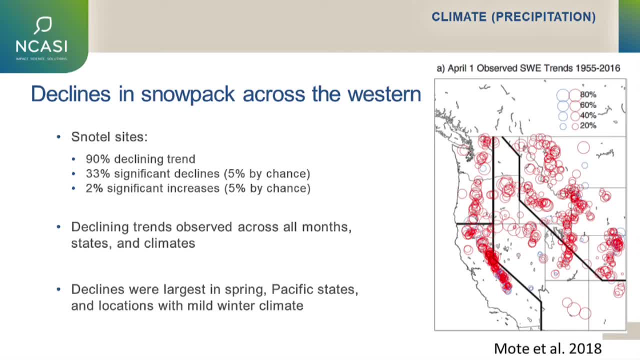 United States and they found that ninety percent of those sites had trends of declining trends of April 1st snow water equivalent, so the amount of snow present on April 1st each year. Of those, 33% of those were significant declines and 2% of sites showed significant 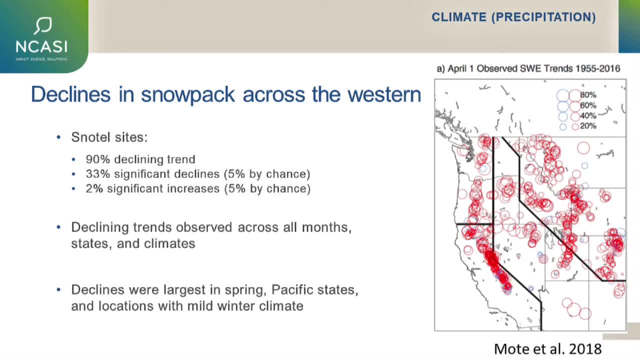 increases On this figure, the red indicates a declining trend and the blue indicates a positive trend. in terms of the spatial variability of those responses, All of those declining trends were observed across all months, states and climates, and the declines were largest in spring in Pacific states and 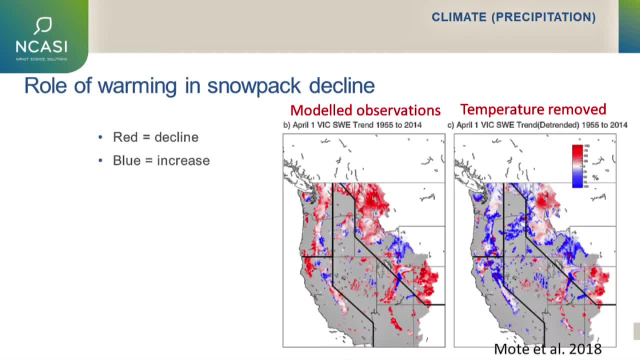 locations with with mild winter climate, Continuing with their results. this is also from their paper, in this case, taking those observations and applying it to a model. On the panel on the left you have those models: observations for April 1st: snow water equivalent On the right. what they've done is they've 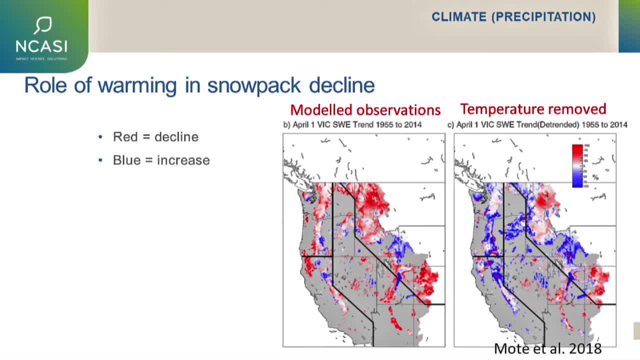 detrended the data set to remove the effect of temperature to evaluate the data set to remove the effect of temperature to evaluate the effect of role of warming on that snowpack decline. And so you can see that on the figure on the right in Oregon and Washington there's no longer large swaths of red. 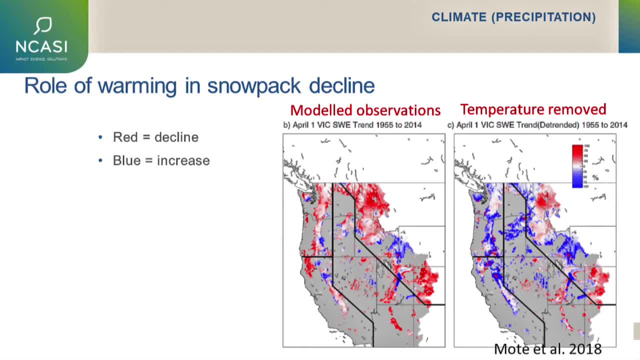 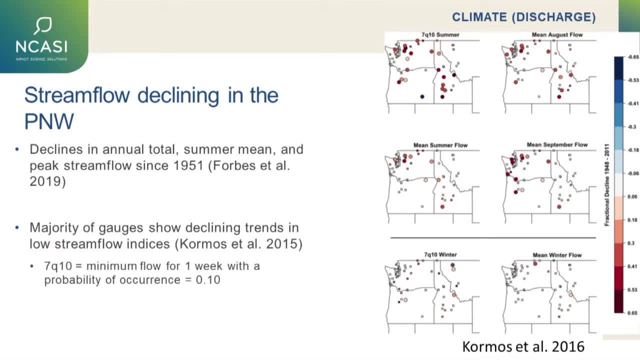 indicating significant declines, as there were prior to the detrending of the temperature response. So, ultimately, being interested in streamflow, streamflow has also been observed to decline in the Pacific Northwest over time. Declines have been observed by multiple studies. Declines have shown: 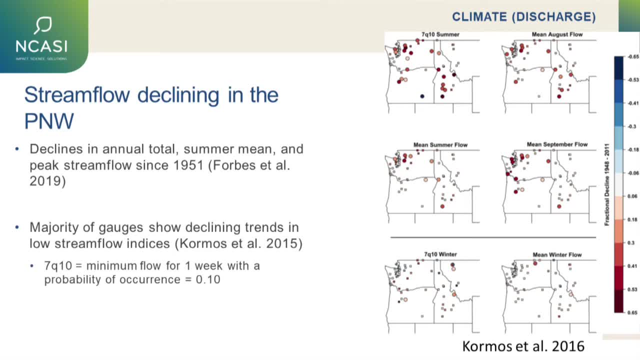 declines in streamflow at annual basis, in terms of mean summer flow and also peak streamflow. In this study, this figure is showing you results from Cormos and others in 2016.. Where they're looking in the top four panels, those are: 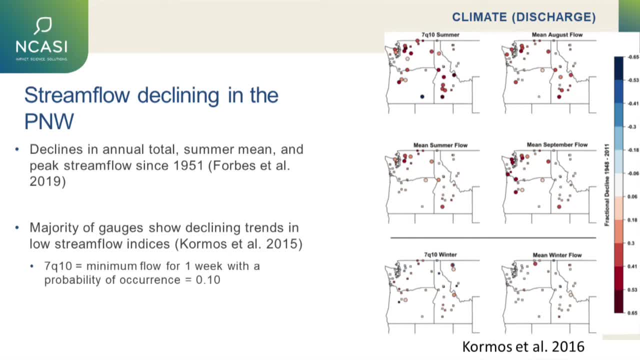 four different metrics of essentially low flow metrics. So those are using a mean August flow, mean September flow, mean summer flow and also an index they're calling the 7Q10, which is minimum flow for one week at the probability of 0.1. 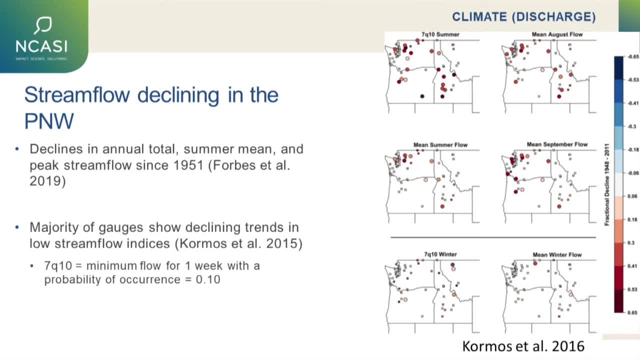 occurrence, And you can see by the red circles that generally there's a decline in those various summer metrics across the Pacific Northwest. The bottom two panels are just showing you similar metrics but for winter, and so there you're not seeing those major declines as 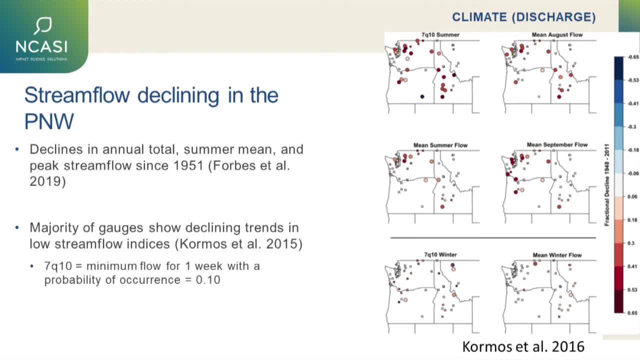 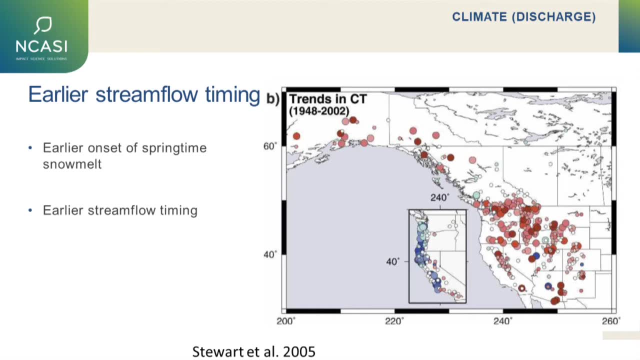 were observed during the summer streamflow season. So, in addition to having declines over time, an earlier analysis also demonstrated that there's earlier streamflow timing And so, as we previously discussed, there's earlier onset of springtime snowmelt, but also observations of earlier streamflow. 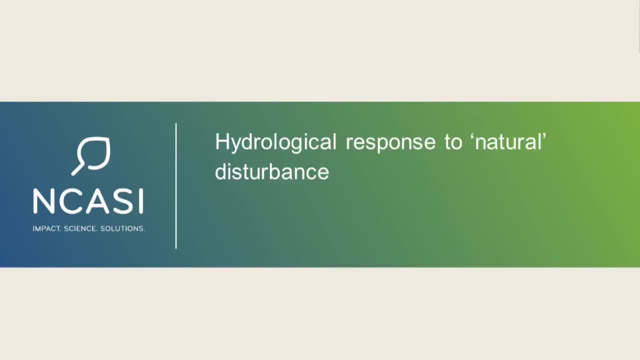 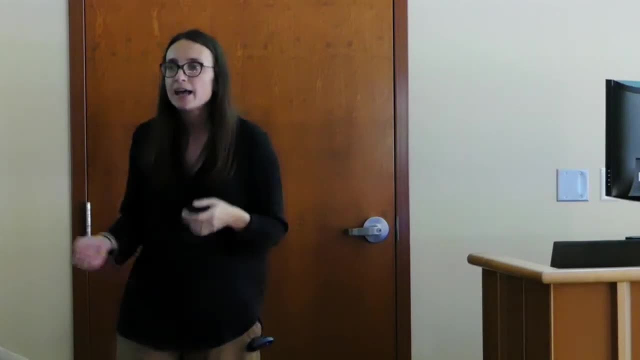 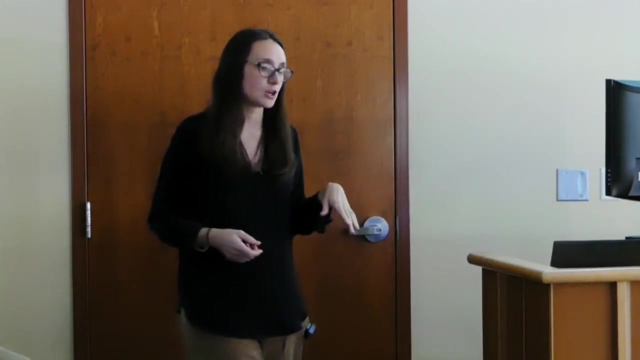 timing. So those are sort of how climate is currently affecting many of those components of the water budget. And now I want to move into talking about what some of the hydrological responses are to some of these natural disturbances that may be related to some of the climate. 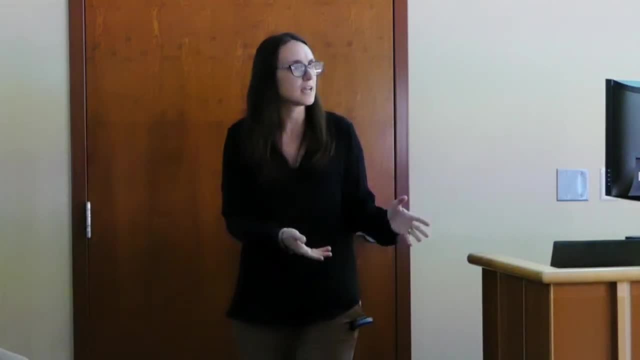 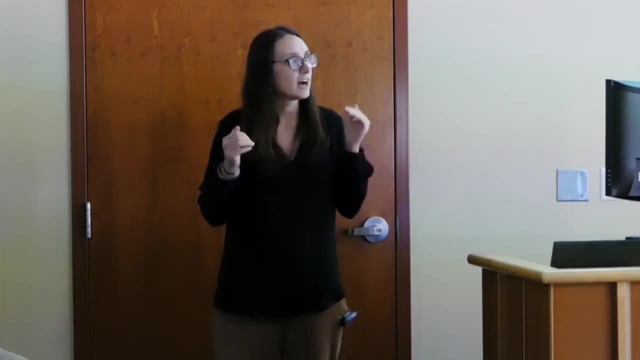 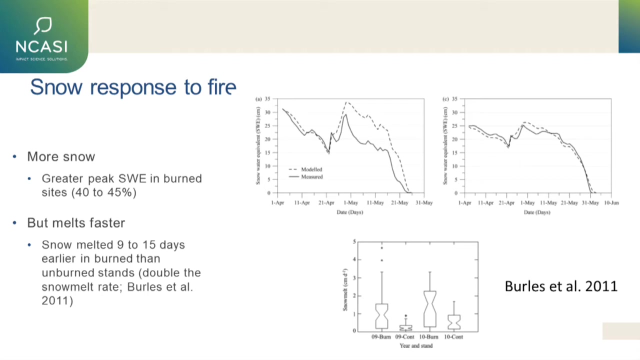 change factors. So we've talked a little bit about fire today and I think there'll be some more discussion about that later, But understanding the fire response, how fire may affect the hydrologic cycle, is important. So, in terms of snowpack, in this study in 2011,, this is a study from Western Canada where they found that 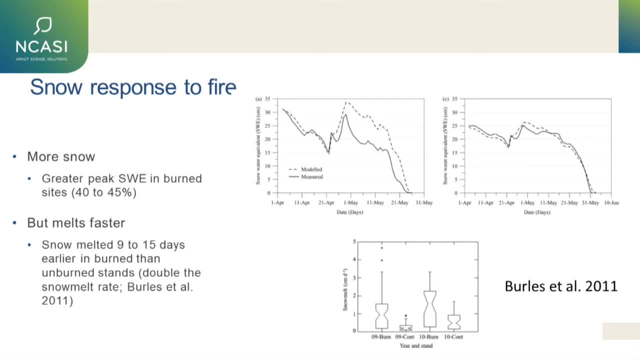 in a burned site- that's the panel on the top left- there was more snow accumulation that occurred at the burn site relative to the control site, which is the site on the right, And so they found that peak snow water equivalent. so the amount of 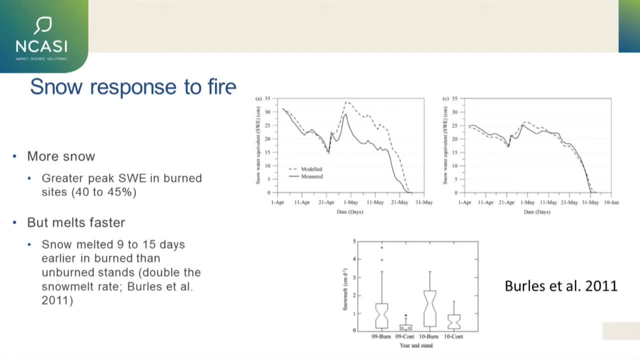 snow was 40 to 45 percent greater in the burned site than the unburned site, So theoretically that's great that there's more snow and potentially more water available. However, they also found that it melted faster, And so it actually melted nine to 15 days earlier in the burned site than 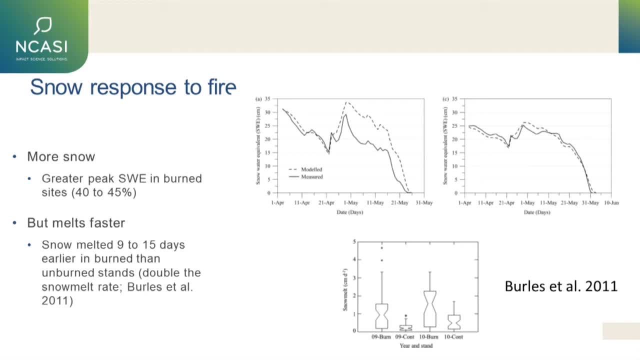 in the unburned site And we'll talk a little bit more about this in terms of observations following clear-cut, which would follow a similar pattern. That panel on the bottom is showing you the snowmelt rate, So the burn are the two. 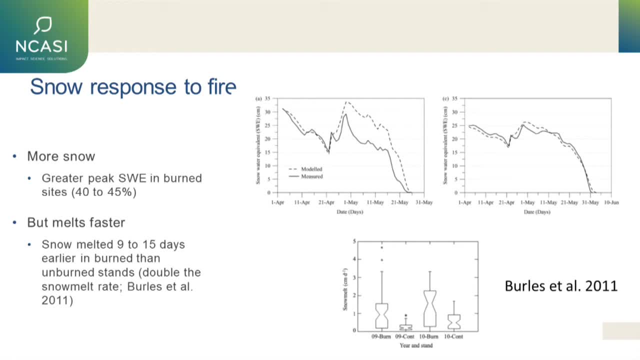 there's two different years that are measured, but it's showing you that the burn, the snowmelt rate is actually double that in the burn stand relative to the control stand. So that's snowmelt response to fire. but streamflow response to fire is also important to. 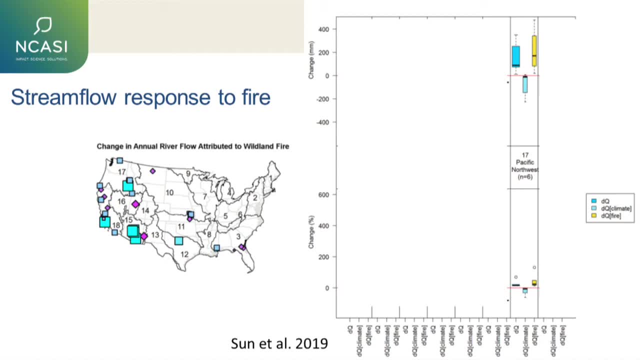 understand, This is a very recent report, drafted by Sun et al in 2019, and if we focus specifically on the Pacific Northwest region, that's region 17.. Here in this figure, the yellow bar on the right is showing you the expected change in discharge attributed to fire, And so the top panel. 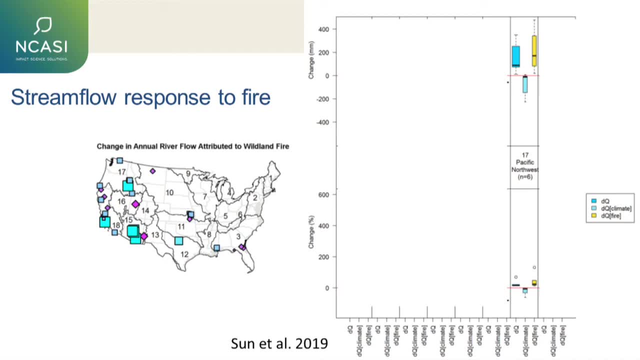 is change in terms of quantity of millimeters and then the bottom panel is change in terms of percentage. So the yellow is showing an increase, The lighter blue, which is the middle bar, is a change in discharge expected due to climate alone, And then the one on the left, the far left, darker blue, is change. 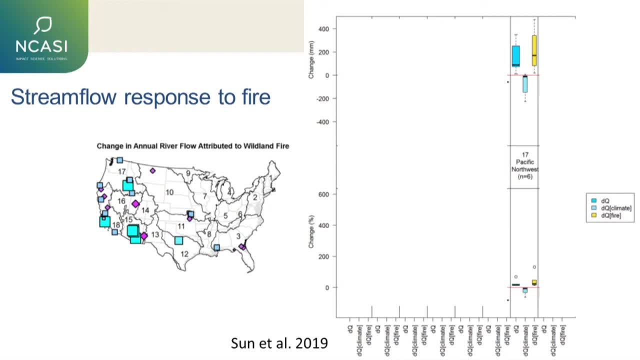 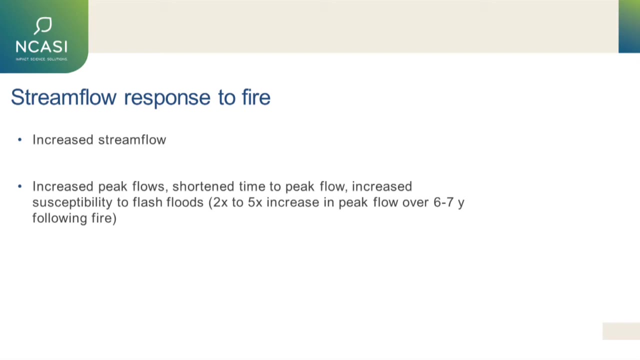 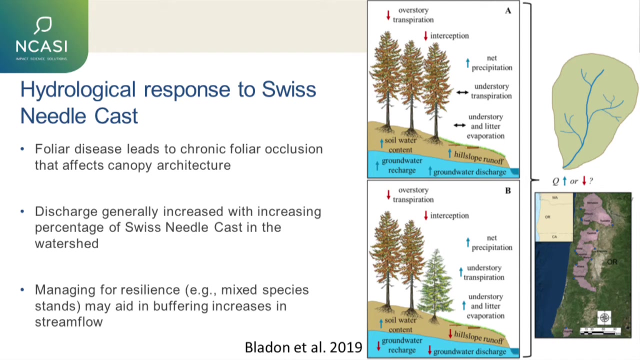 in discharge due to both processes. So fire plus climate still indicates a positive change expected for region 17 in their analysis. So just to rehash those findings, there's anticipated increased streamflow with fire, including increased peak flows, shortened times to peak flows and increased susceptibility to flash floods following fire. So I only 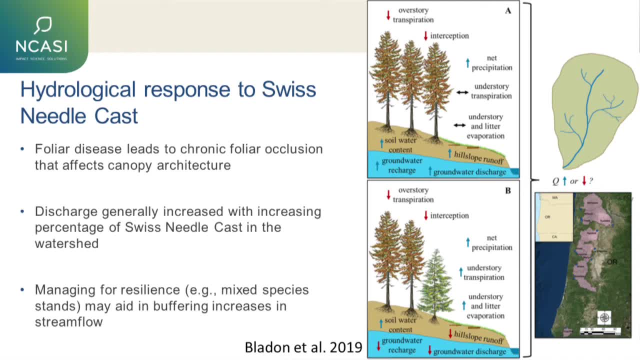 have one example of this, but it's a very. it's a good example of understanding what some of the forest pathogens may do in terms of affecting forest hydrology. Kevin Bladen and his collaborators at Oregon State University recently published this in Science of the Total Environment. So 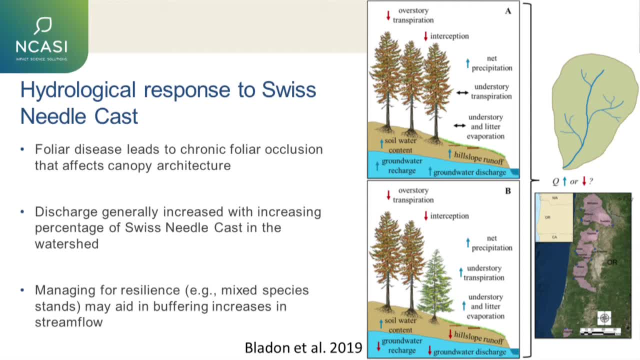 they looked at Swiss needle cast, which is a foliar disease that affects Douglas fir, and it can lead to chronic foliar occlusion that affects canopy architecture and affects, of course, transpiration rates in those systems, And so you might hypothesize that that 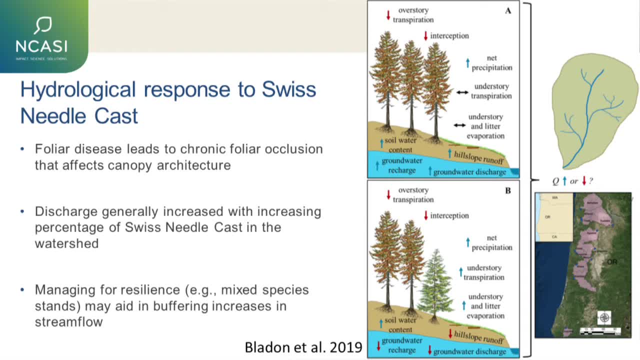 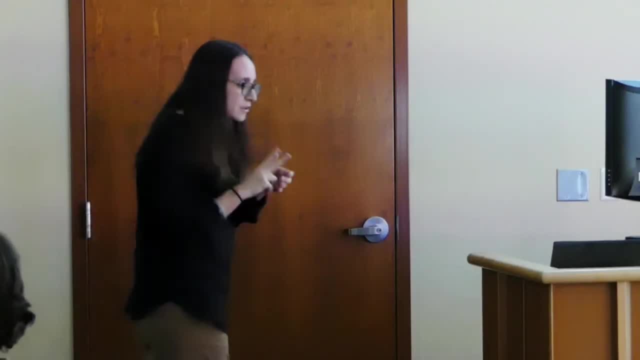 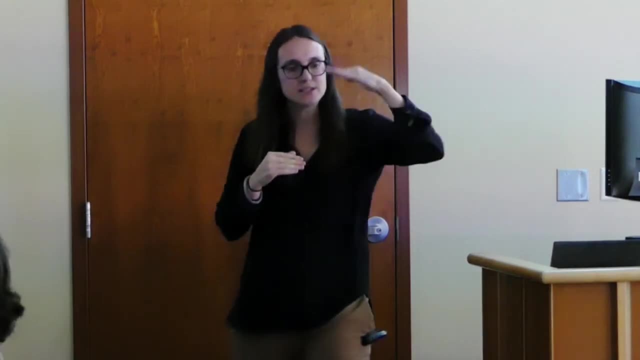 trees affected with this would have lower transpiration rates, which would mean greater water availability, greater runoff for the ecosystem itself. So that's one hypothesis. However, based on other literature- there's from, I think, Pine Beetle- they found that even though there was depressed, 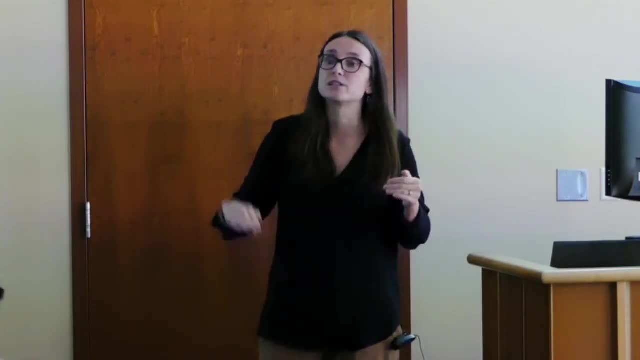 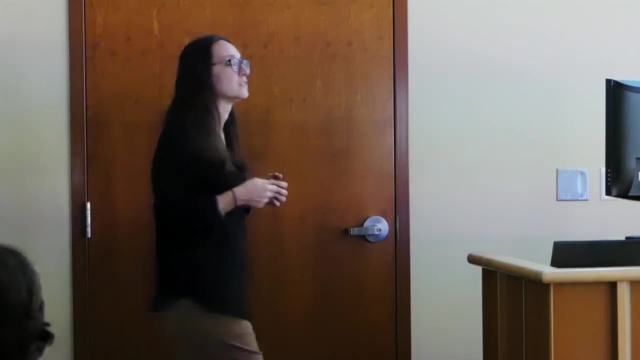 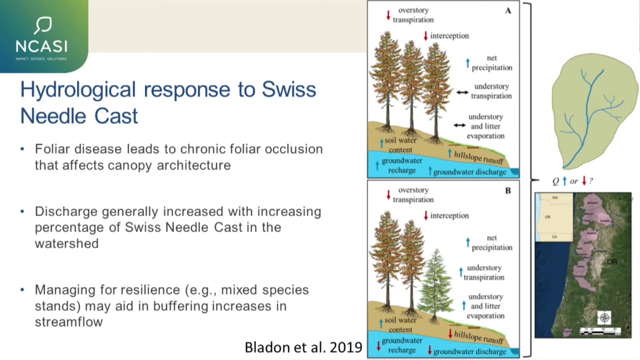 transpiration rates. there was actually an increase in evaporation and transpiration of understory vegetation and other surfaces. that sort of counterbalanced that. so they didn't actually see an increase in runoff. So in this particular study what they did find, they used a gradient across Oregon of a 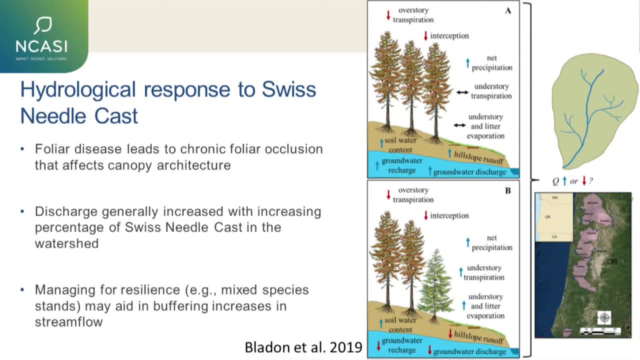 variety of sites and they found that discharge did generally increase with increasing percentage of Swiss needle cast in the watershed. And then they posed these two scenarios, top panel A and bottom panel B, to determine the Fuji's evaporation response in terms of what that expected hydrologic. 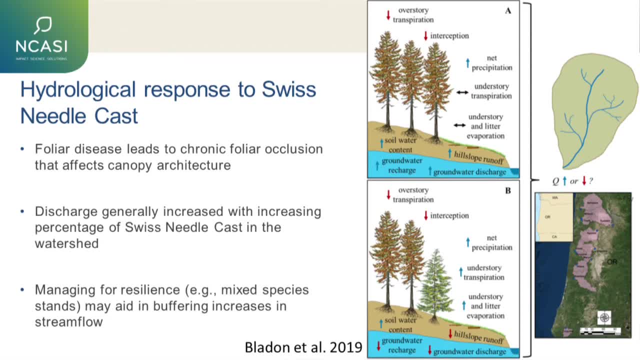 response might be with the top panel showing you a monoculture Douglas fir complete with all of them affected by Swiss needle cast, And that top panel primarily differs from the bottom panel in terms of that understory transpiration component and also the understory and litter evaporation. 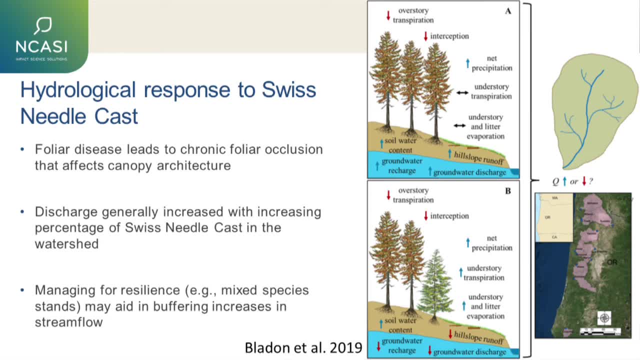 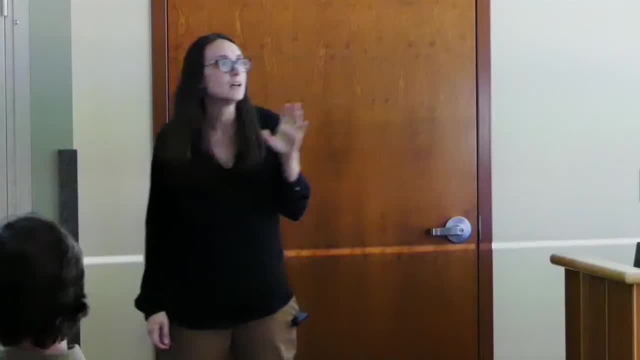 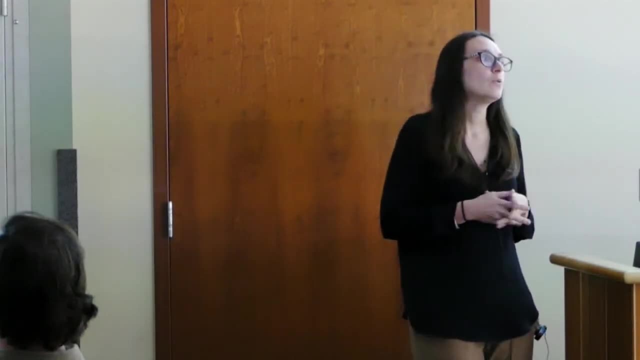 component. So no change in panel A which ultimately results in increased surface runoff in panel B and Apollo e- be when they have additional species present. So while transpiration does decline, they also see an increase in understory transpiration, an increase in understory and litter evaporation, which 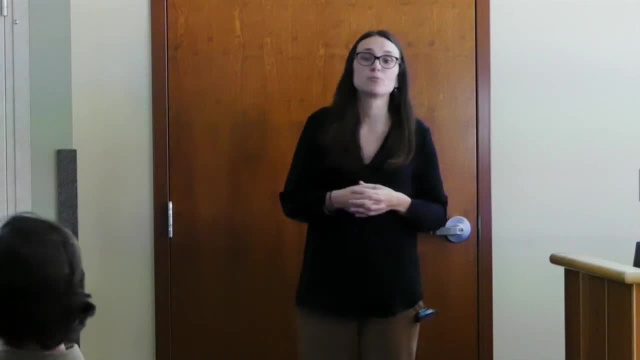 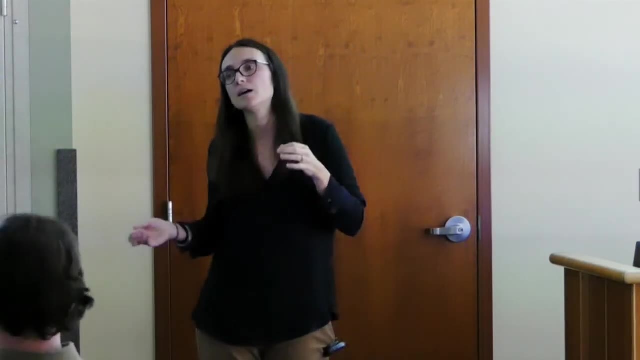 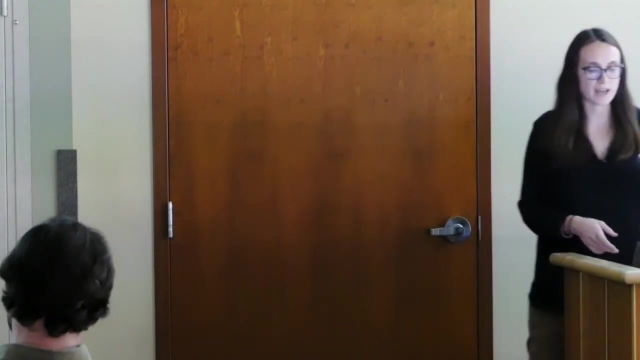 ultimately can maybe reduce the hill slope runoff, But overall, based on their findings, they recommended managing for resilience by incorporating mixed species stands. that may aid in buffering increases in stream flow in places where Swiss needle cast is a concern. So now I'm going to move into what 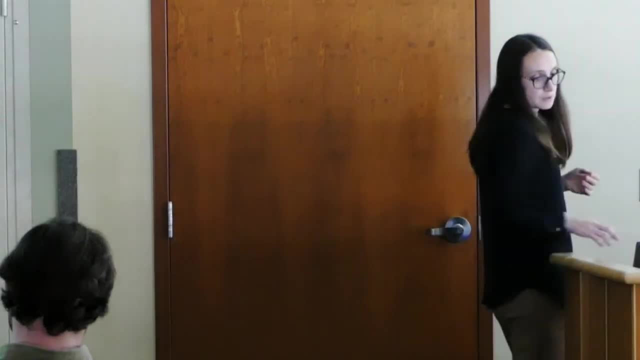 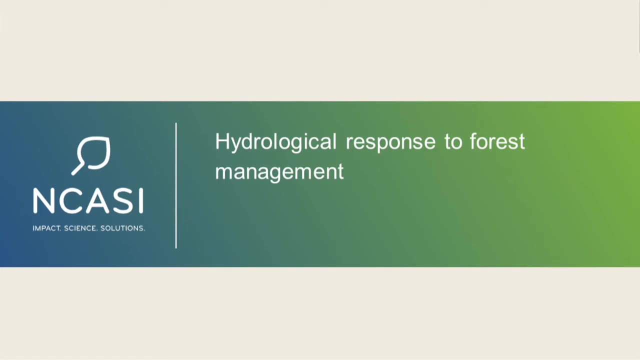 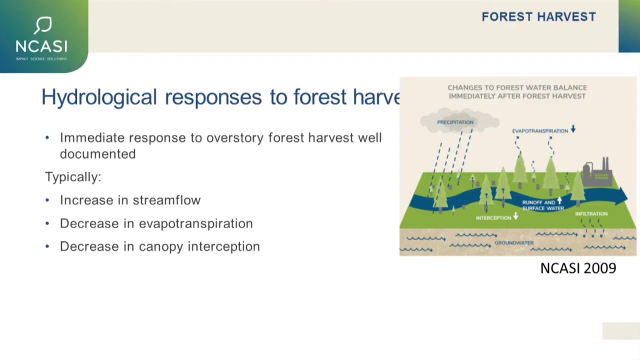 some of those hydrologic responses are to forest management. So the hydrological response to forest management is well studied. There are hundreds of paired watershed studies that have evaluated the immediate response to overstory removal, And so this figure on the right is a figure based on the generalized response. 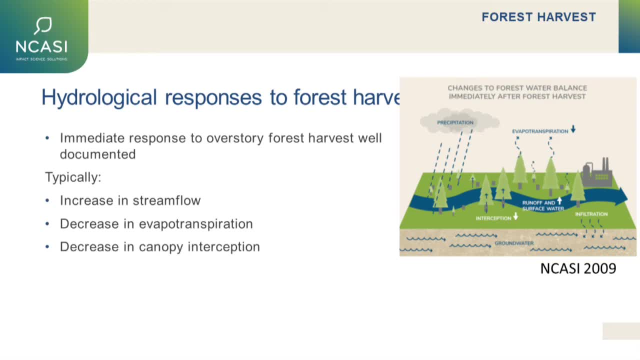 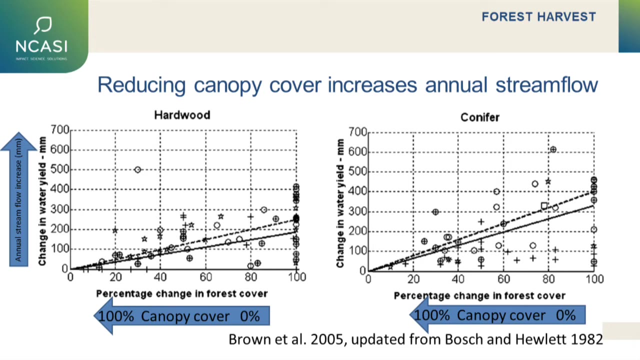 of a broad spatial areas, which are generally that when you remove large swaths of overstory vegetation, you have an increase in surface runoff, you have a decrease in evapotranspiration and you have a decrease in canopy interception. To demonstrate some of these, 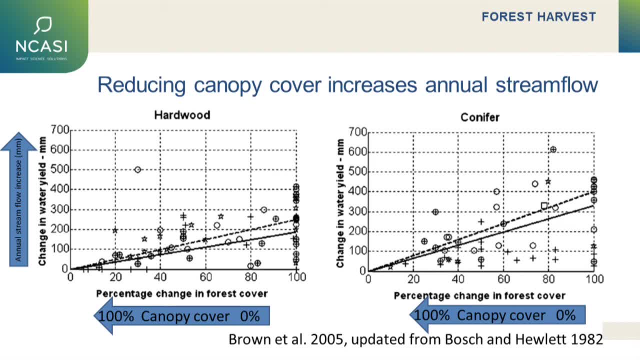 To demonstrate some of these, This is an updated review from Brown and others, which updates the original Bosch and Hewlett findings, which are that reducing canopy cover does increase annual stream flow, And this is true for both hardwoods and conifers, And so that's the immediate response to forest harvest. 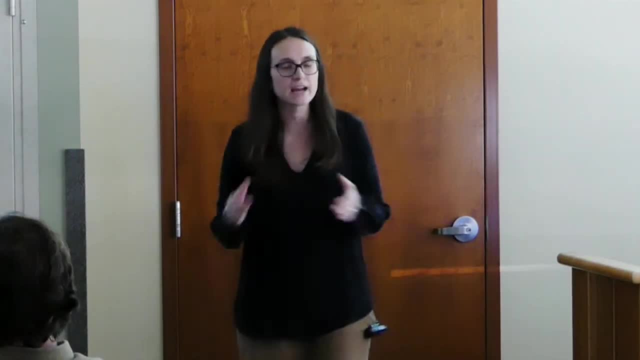 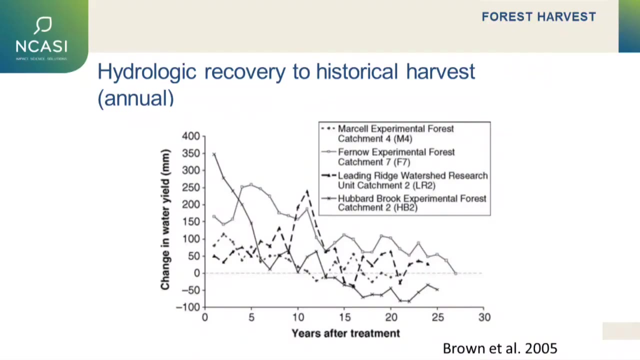 But of course it's important to consider what the hydrologic response is over the course of the entire rotation age, so up to 40 years, 60 years, et cetera. So this is a figure that evaluates that long-term response at an annual basis. 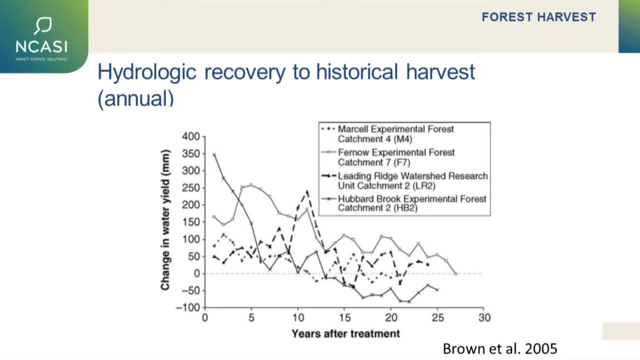 across many experimental forests in the United States. Many of these are deciduous species, So I wanted to point out that basically, the expected response is that immediately there's an increase in flow And then, as green-up occurs, then you start to see this hydrologic recovery. 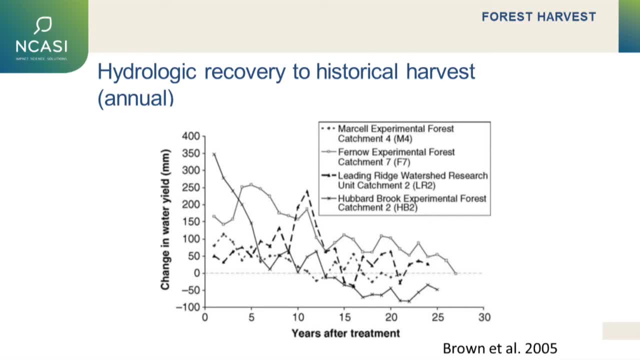 And so you can have this variable period of discharge response as that's being recovered. But ultimately, as those ET rates continue to increase, you may begin to see a deficit in terms of the hydrologic budget at some sites overall. And so, to demonstrate that this is a figure, 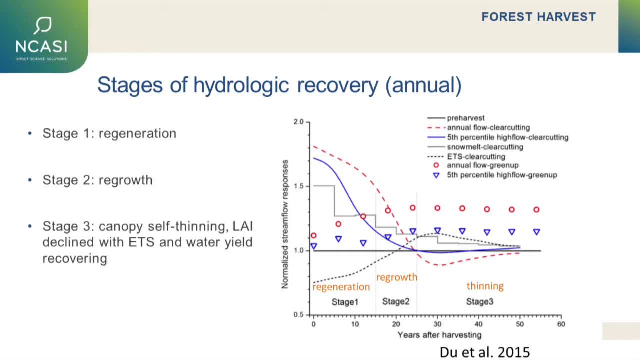 This is taken from a hydrological model of Micah Creek Watershed in Idaho, So I want you to look specifically at the red dashed line. So that is the modeled response And you can see that the hydrologic response is the same as the hydrologic response to annual flow. 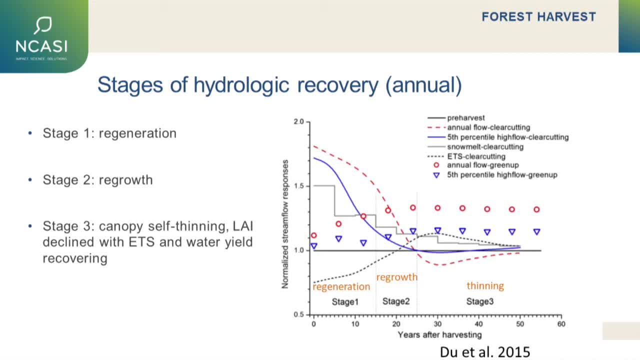 clear-cutting of 100% of the watershed, And so what that demonstrates is that, yes, you see that expected increase in annual flow during stage one, And so they've defined that stage one is that regeneration period. If you look at the red circles, those 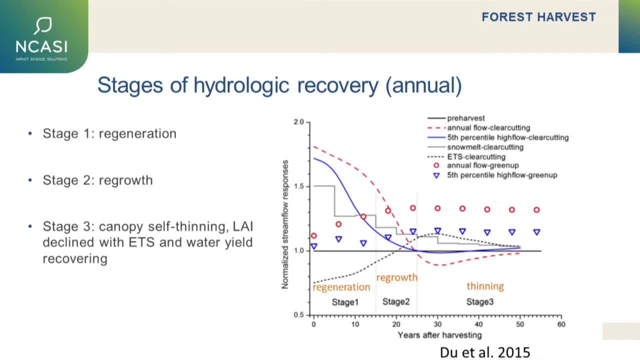 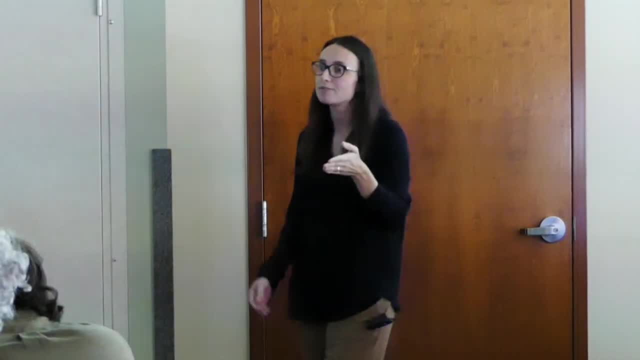 indicate the green-up and how that's changing over time So you can evaluate sort of what the hydrologic response looks like in relation to the green-up period. So during stage two, as you have that regrowth, that's where you have that hydrologic recovery or return. 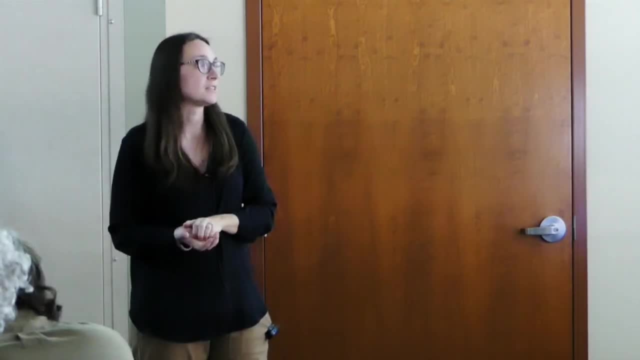 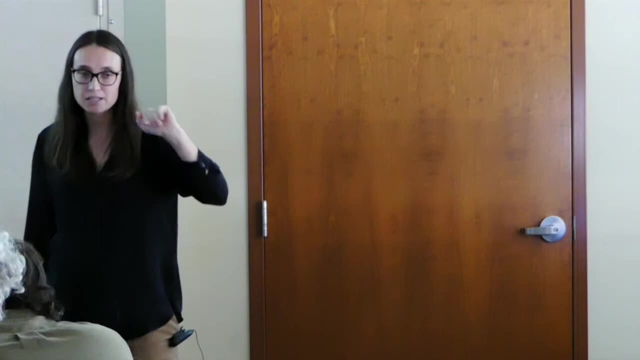 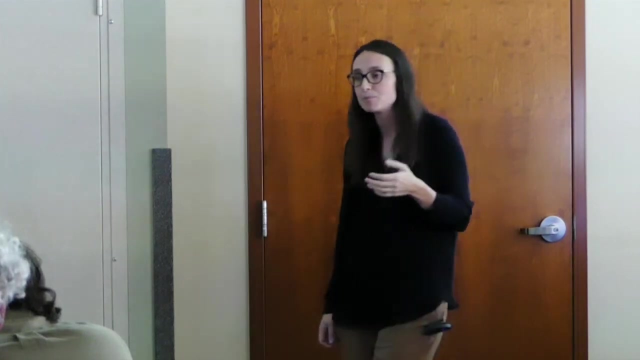 to baseline conditions in terms of that overall response. They then see the undershoot response. So this is where there starts to become a deficit in terms of annual flow And then in their model, their model underwent a canopy self-thinning which allowed that hydrologic response to return. 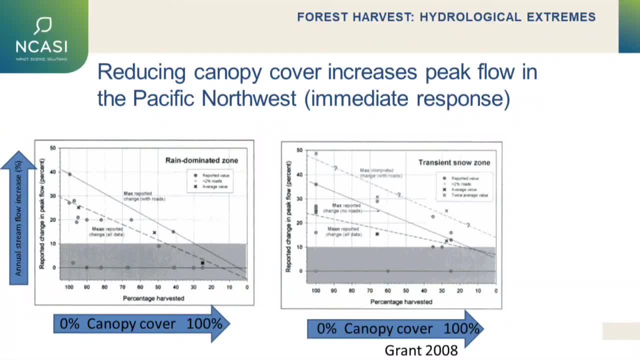 to those baseline conditions. So those are some examples. Those are annual flow responses, But of course understanding those hydrologic extremes are also very important. So if we look specifically at peak flow responses, the peak flow response does follow the same trend as annual responses, which are that reducing cover. 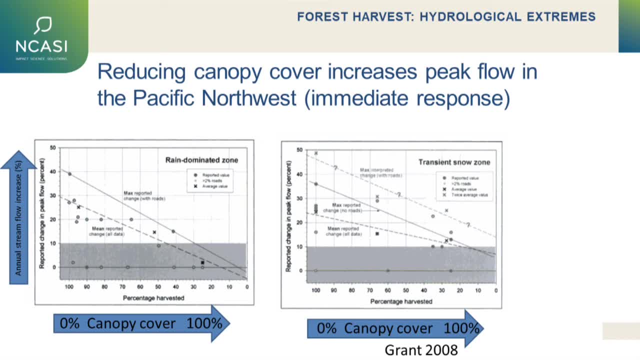 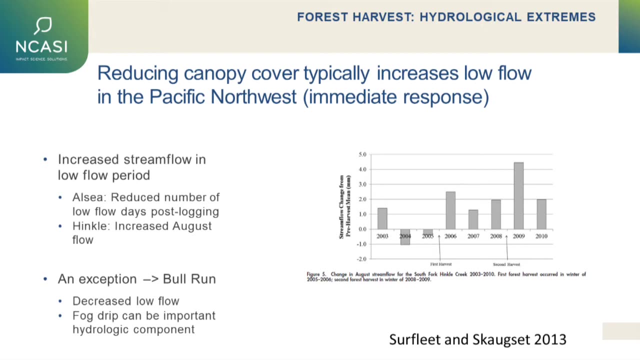 does increase peak flow And this particular review is specific to the Pacific Northwest And, again, this is the immediate response to that removal of vegetation In terms of the low flow response. also the same directionality in terms of a response immediately after harvest. 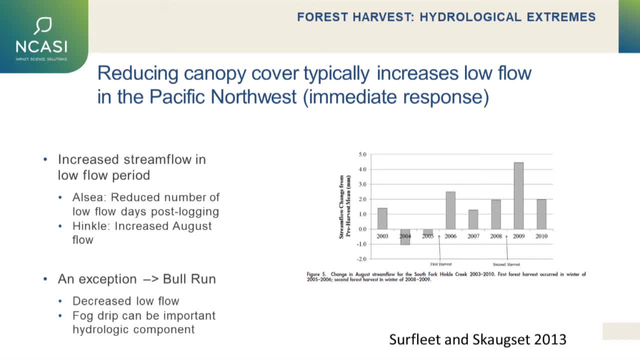 In the original Alsea watershed study they did find a reduced number of low flow days. that occurred immediately post-logging And then also more recently following. the recent contemporary paired watershed study at Hinkle Creek, Surfleet and Skagset have observed in mean August flow an increase following those. 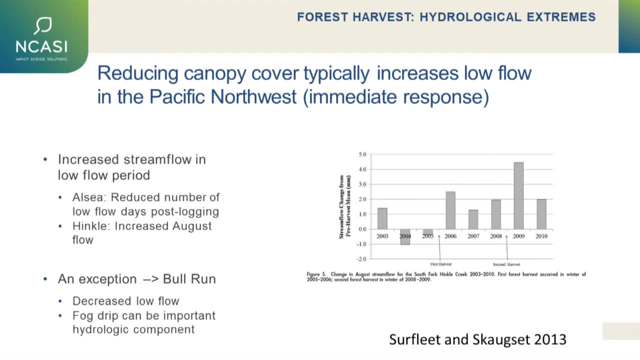 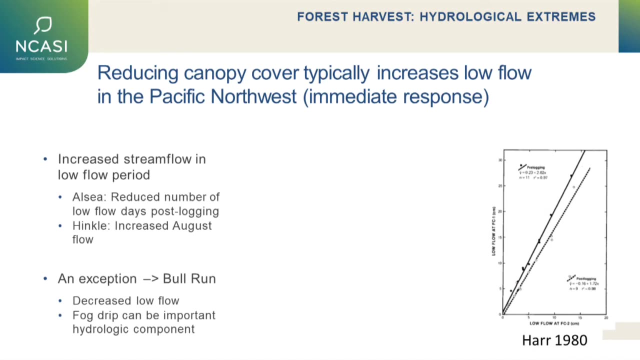 two harvest periods, So those little arrows are representing two separate harvest events that occurred And you can see that the year immediately following those events there was an increase in those low flow metrics. One exception to this is Bull Run watershed, where Haar in 1980 found that there was actually 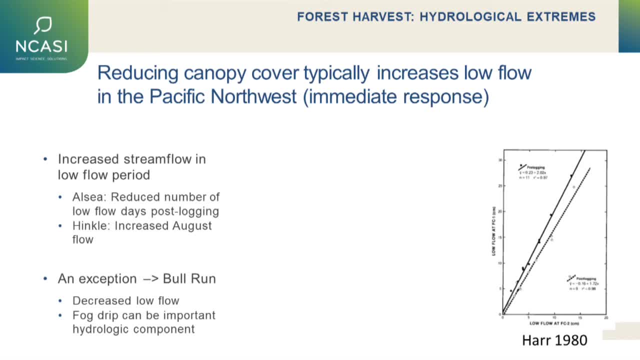 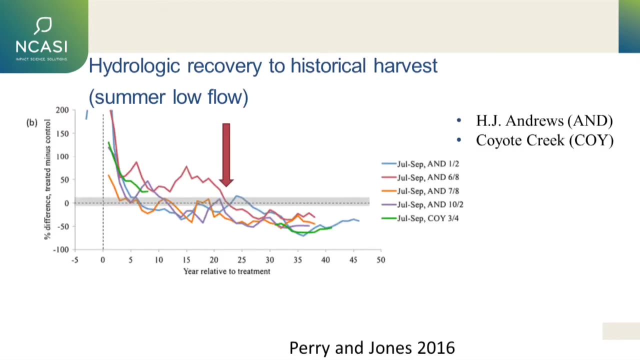 decreased low flow immediately after harvest And they were able to attribute that to fog drip, which is a very important component of the hydrologic budget in that particular watershed. So we talked about the long term response at an annual scale, but also we can look at that at a low flow scale. 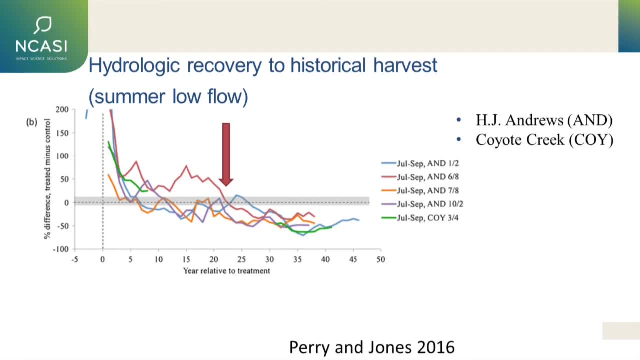 So this is a figure from Perry and Jones 2016,, where they evaluated streamflow response at HJ Andrews and Coyote Creek, both of which are in Oregon, in the Cascades, And so they saw the same general trends where there's. 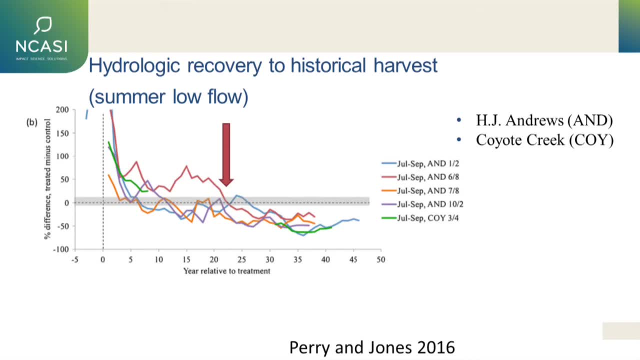 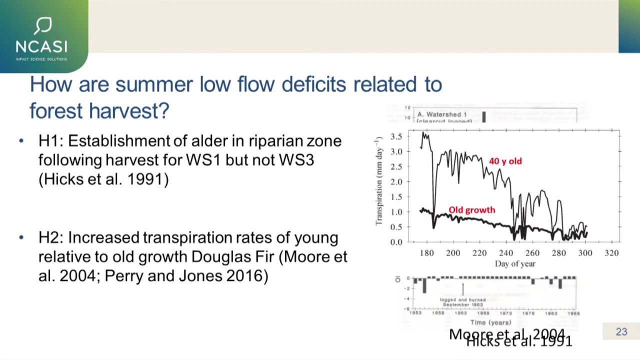 an increase in flow immediately post-harvest. There's some variable recovery period with a return to baseline, But then after 20 years they start to see these deficits across the sites that were evaluated. So how are those summer low flow deficits related to forest harvest? 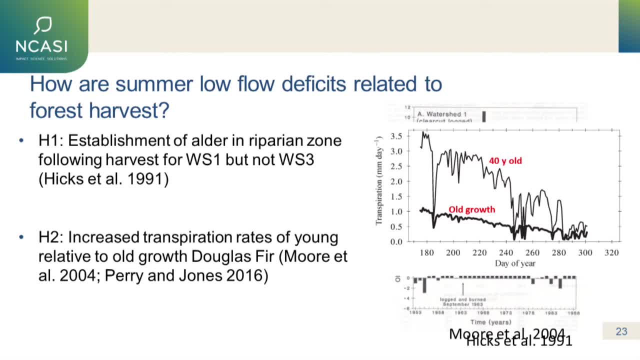 When this was originally observed at the HJ Andrews. the top panel here is watershed One and you're seeing those deficits that occur following harvest. They hypothesized that this was due to establishment of alder in the riparian zone at watershed one, which 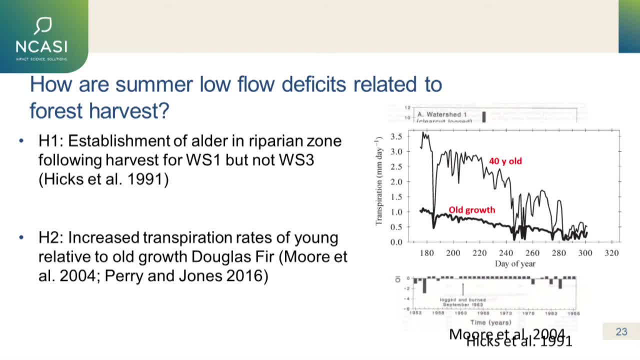 did not occur at watershed three, Of course, watersheds one and three. watershed one was 100% clear cut. Watershed three was 25% patch cut, And so the hypothesis is that it's conversion from primarily coniferous old growth to a deciduous tree. 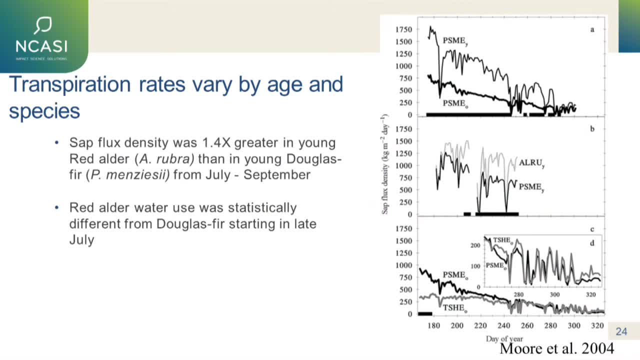 species. The more recent hypothesis is that it's attributed primarily to stand age, And so the increased transpiration rates of young relative to old growth, Douglas fir, are also a leading hypothesis. So this figure is a figure from Moore's 2004 paper. 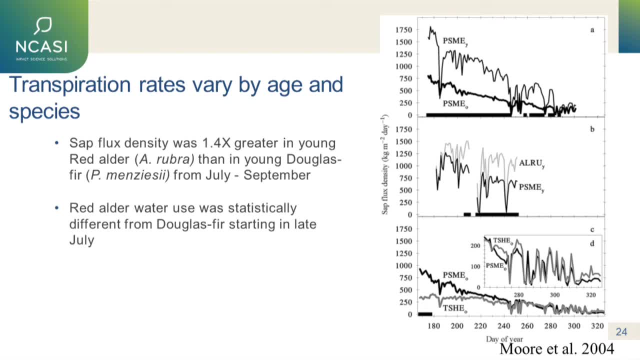 where they did SEPFLUX measurements to look at transpiration rates, You can see that the transpiration rate of the 40 year Trees is much greater than an old growth tree. And then if we look at some additional information from that paper now we're moving. 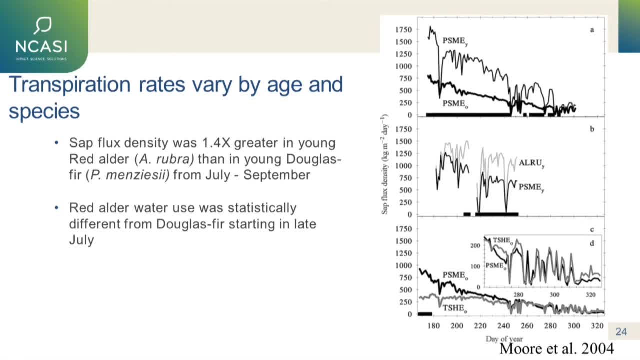 where the y-axis represents SEPFLUX density as opposed to transpiration rate, And so that top panel is essentially the same figure as what we just looked at. If you move into the middle figure here we see young Douglas fir, SEPFLUX density, and then above. 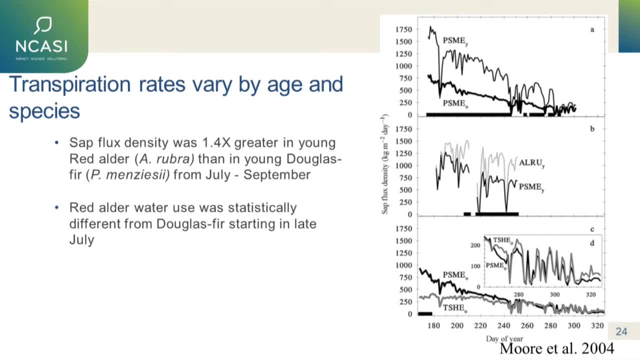 that is the red alder. young stand SEPFLUX density. And so they did find that SEPFLUX density was greater in red alder than Douglas fir and that it became statistically different, beginning in late July and continuing through the growing season, as you can see there in panel B. So certainly 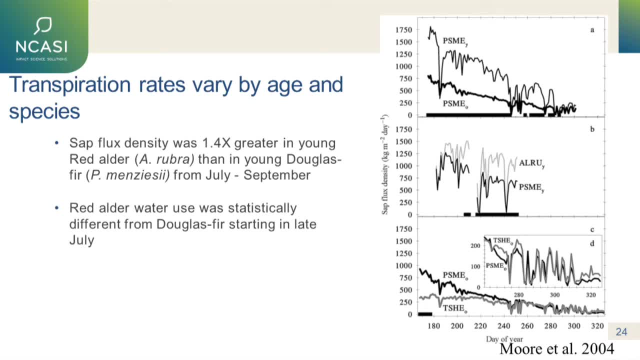 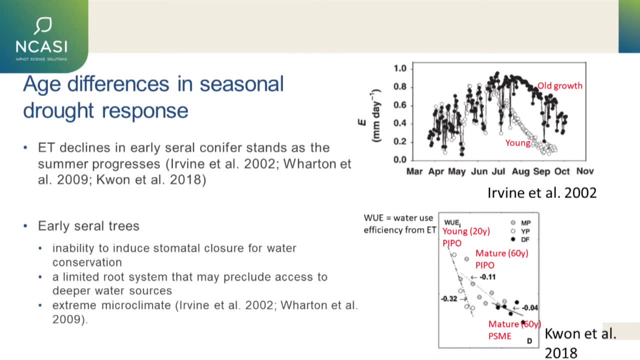 transpiration rates do vary by age, but also by species. There are also age differences, And so in the seasonal drought response, and so this is a response that's been widely observed through a variety of eddy covariance measurements throughout the Pacific Northwest- 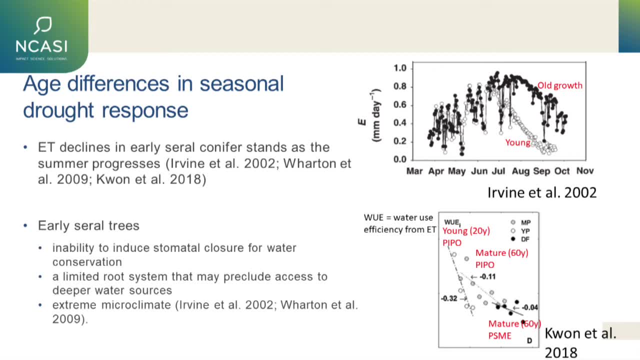 So three studies cited here did find evapotranspiration declines in early sterile conifer stands relative to old growth. This top figure on the top right shows that separation, as you move into the growing season, into summer, of how old growth responds relative to young. 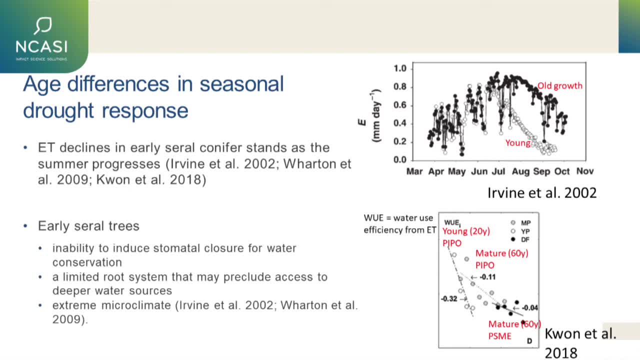 And these are eddy covariance measurements, So these are sort of actual evapotranspiration. So it's not just transpiration, This is the entire ecosystem's response, So that incorporates the old growth stands are not just a single species. There are, I believe, eight species of conifer and three species. 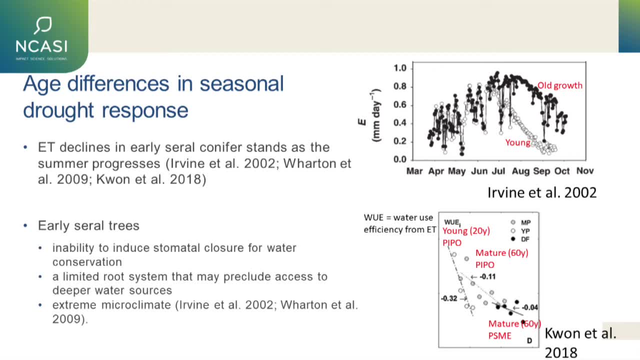 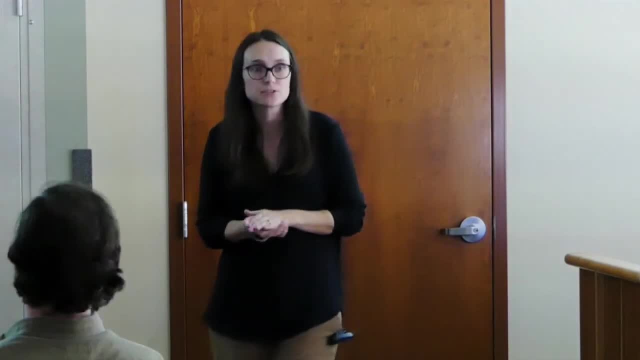 of deciduous trees represented here, as well as any understory of vegetation that may be present at either site. So it's hypothesized that this response of early sterile trees is due to the inability to grow, The ability to induce stomatal closure for water conservation. 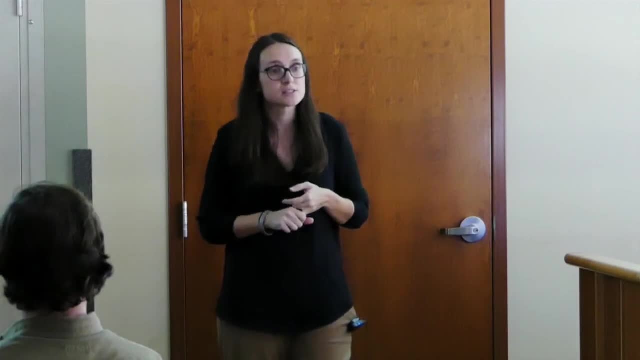 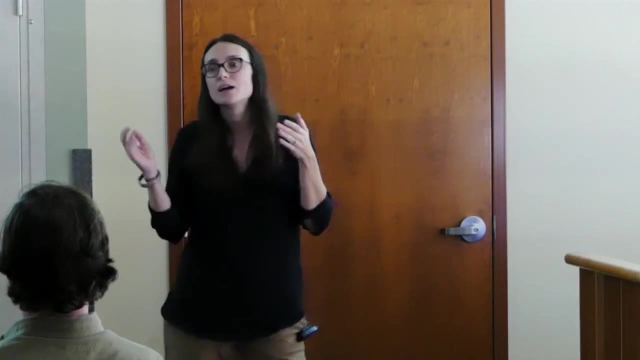 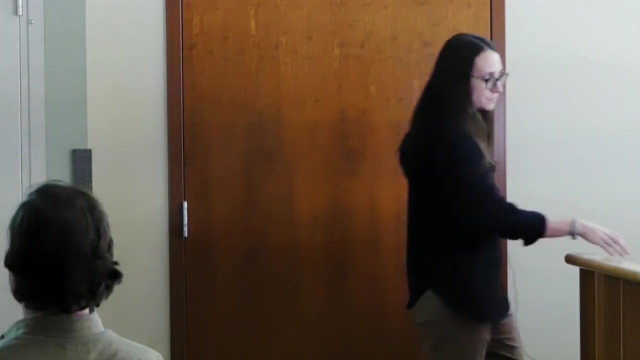 during that drought season, but also a limited root system that may preclude any access to deeper water sources, And then finally, also extreme microclimate conditions that may be faced by some of those younger, early sterile stands. So now I want to move into talking a little bit. 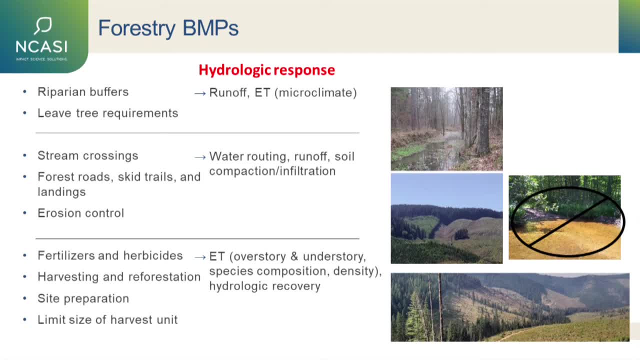 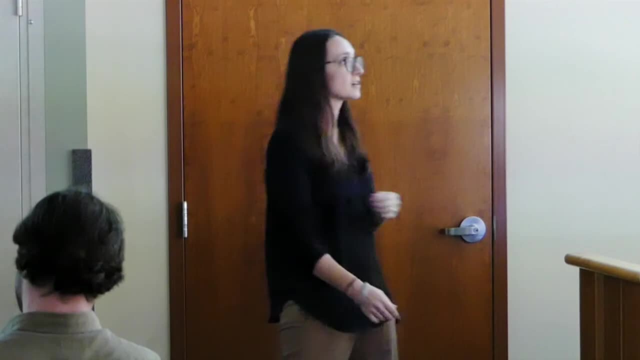 about forestry best management practices. We use the term best management practices because they aren't regulatory everywhere. Certainly, in the Pacific Northwest many of these are regulatory And these are just an example of many of the more commonly applied best management practices, But of course there are many that likely contribute. 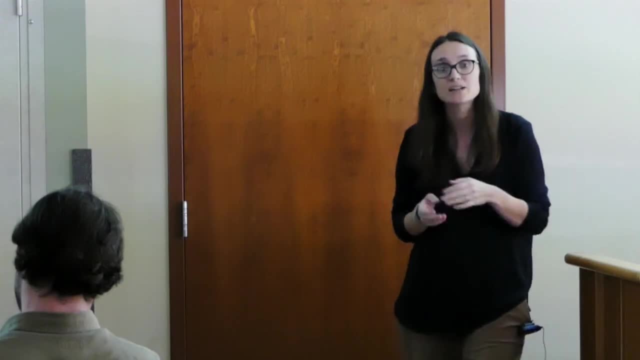 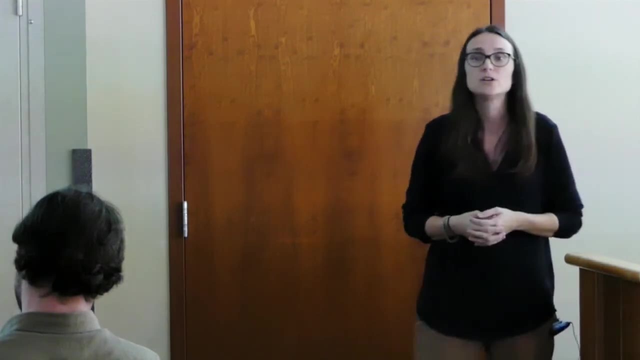 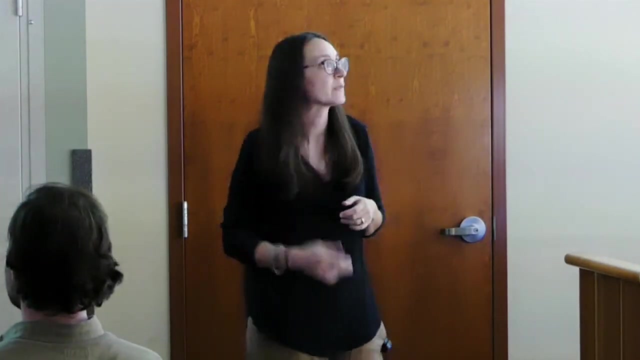 to reducing the hydrological impact based off of some of what those earlier studies have shown, And so many of those paired watershed studies are based on historical harvesting practices And may not reflect contemporary management, particularly when we think about the long term response over time. 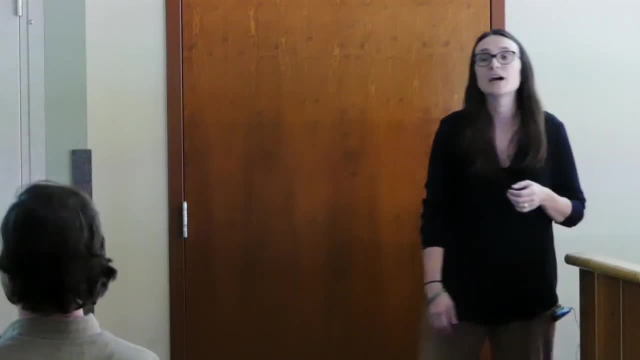 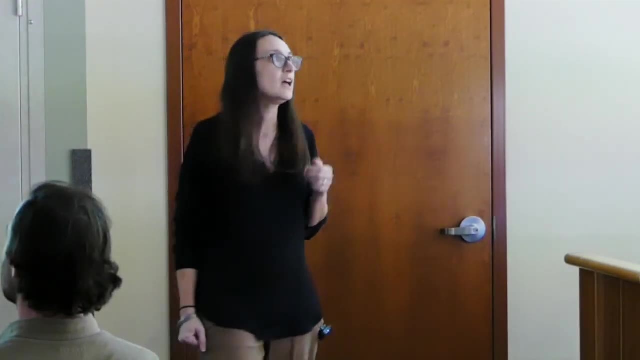 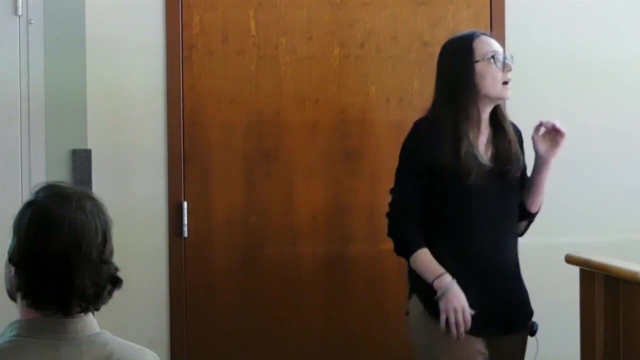 And so, in terms of riparian buffers and leaf tree requirements, those are some of the most widely implemented best management practices across the US and across the globe, And those have very important implications in terms of the runoff component as well as the evapotranspiration component. 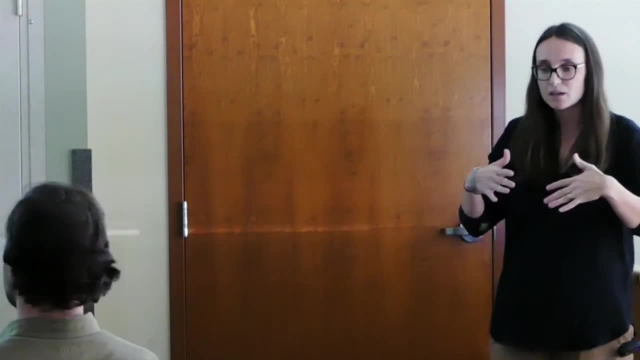 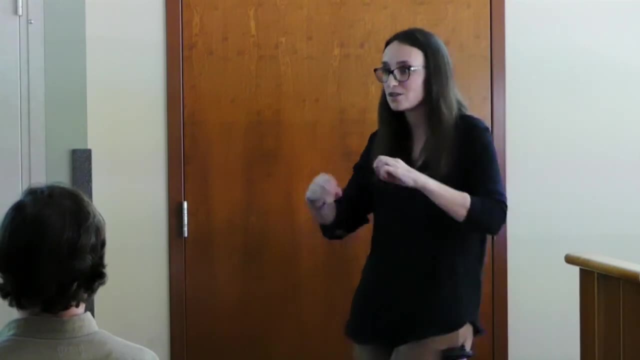 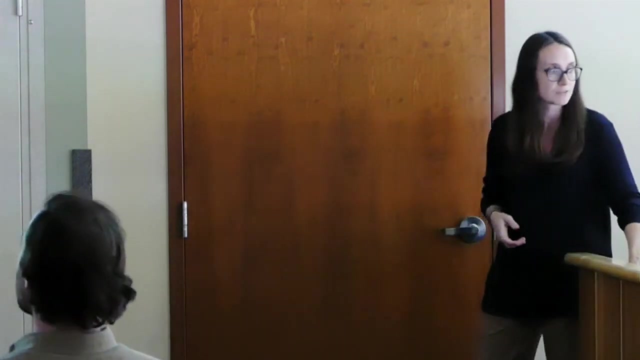 Riparian buffers are particularly interesting as we think about right now. maybe they're 60 or 70 years old, but as those are left and left untouched, then those will eventually become old growth stands that may have very different microclimatic conditions that are important for watershed functions. 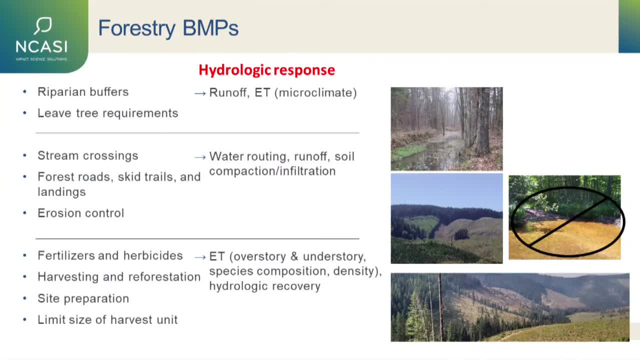 Other best management practices like stream crossings, forest roads, skid trails and landings, as well as erosion control. All of these are important for water routing, And so that's particularly important when we talk about peak flows or storm events, And so that's really important. 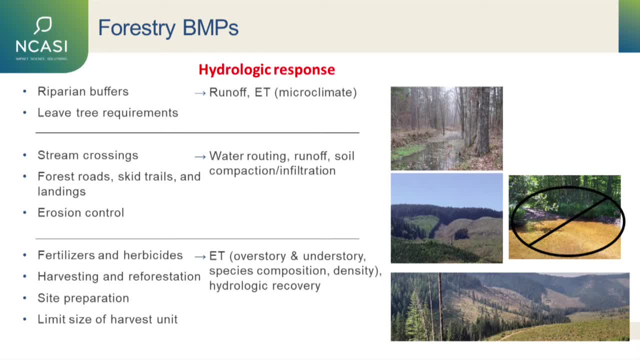 So that's the first thing that we're going to talk about is the soil mitigation. So that affects runoff. Anything that reduces the soil compaction is beneficial in terms of thinking about soil infiltration and, ultimately, runoff. And then there's a variety of other things, including: 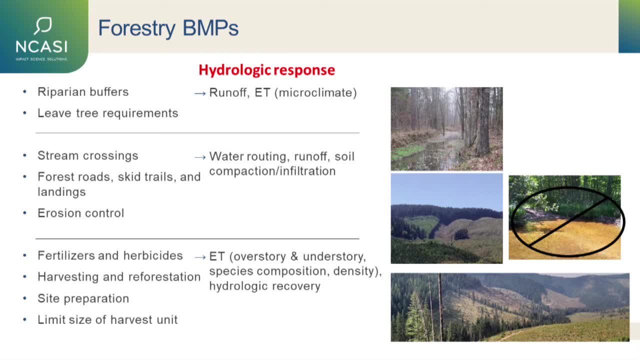 fertilizers and herbicides, harvesting and reforestation, site prep and limiting sizes of harvest units, and so on. And then the second thing that we're going to talk about is the soil management. So soil management has important implications in terms of evapotranspiration rates. 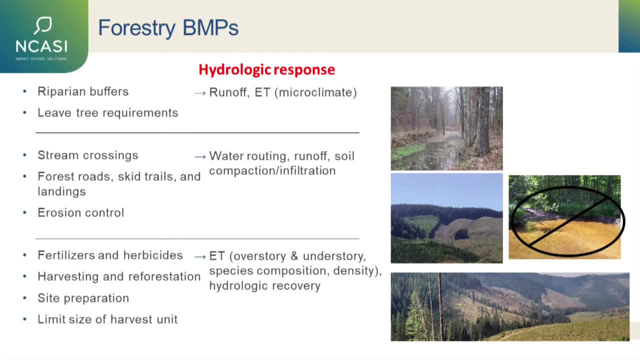 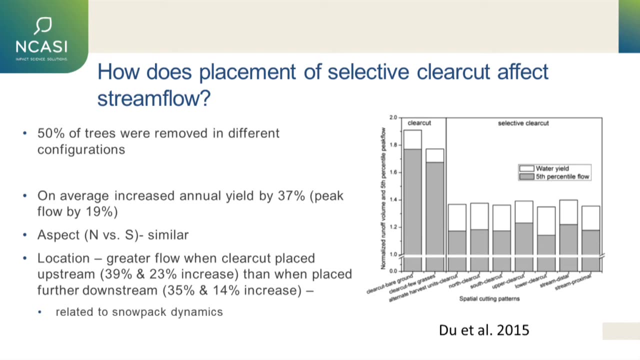 And so that's thinking about this ecosystem as a whole of overstory and understory responses, species composition, density and overall hydrologic recovery over the course of the entire rotation. So it's difficult to tease apart the effects of any one of those best management practices. 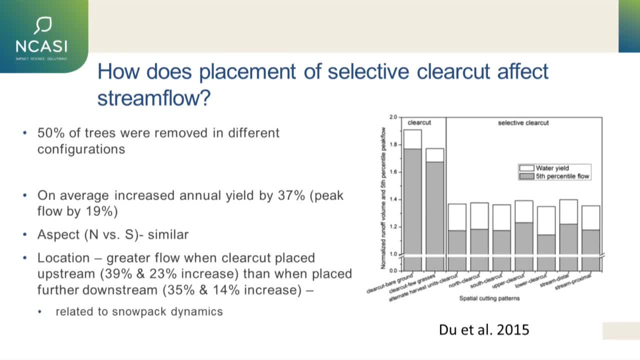 One effort did use their model to look at the effects of 100% clear cut on the watershed and then related to green up requirements, where they're harvesting only 50% of the watershed And so they're taking that placement of 50% harvest. 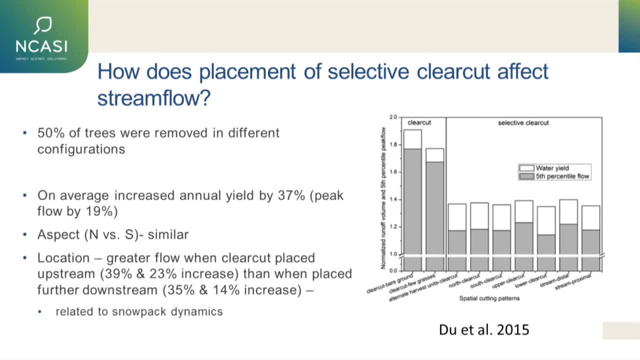 and placing it in different locations within the watershed to try to determine what those effects look like. So on the left you can see the two 100% clear cut responses And then on the right are those selective clear cut responses. They found that when they varied the aspect of the positioning, 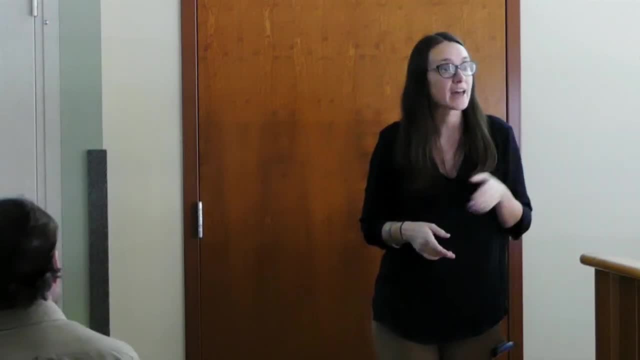 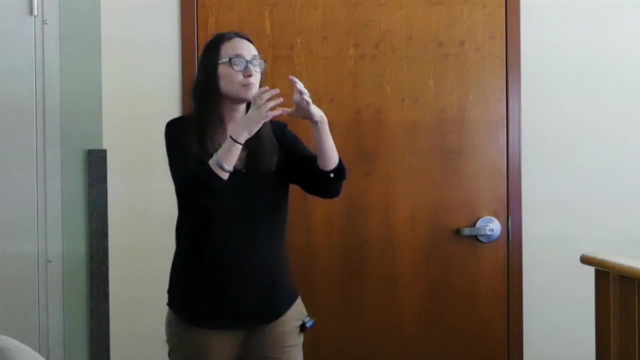 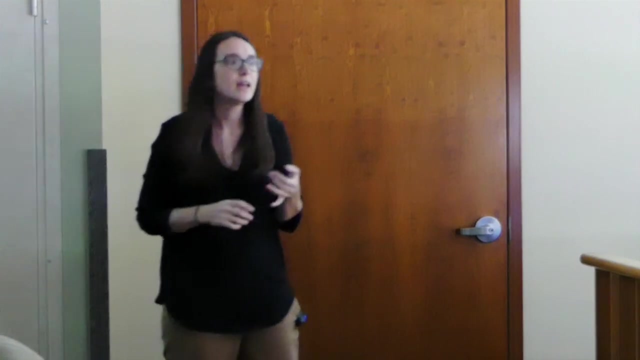 of that clear cut. there was no difference. So it didn't matter whether it was the north aspect or south aspect in their model. But they did find that when they placed the clear cut higher upstream in the watershed that there was greater flow than when they placed it further downstream in the watershed. 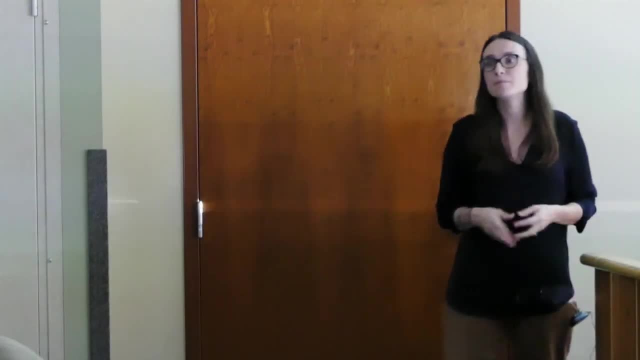 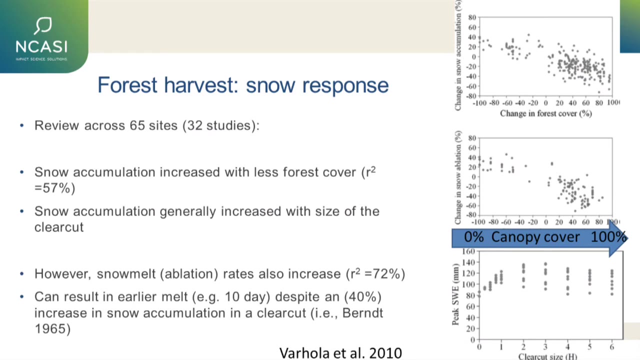 And they have enough data to be able to determine that that's primarily related to snowpack dynamics and elevational changes within their watershed. So, moving into snowpack dynamics, So this ties back into what we observed earlier for the post-fire response in terms of snowpack. 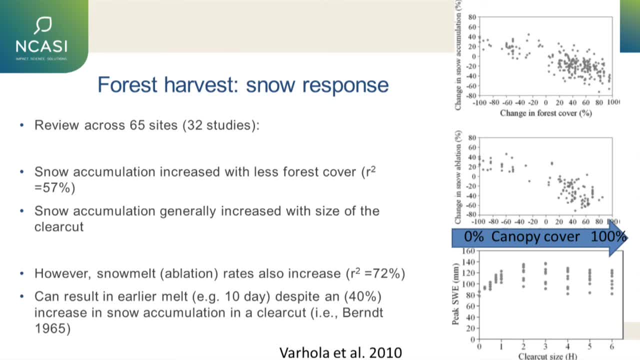 A review of 65 sites, including 32 studies across the globe, has shown that as you change forest cover, as forest cover increases, you have less snow accumulation that occurs, And so, with a clear cut, this bottom panel shows clear cut size. 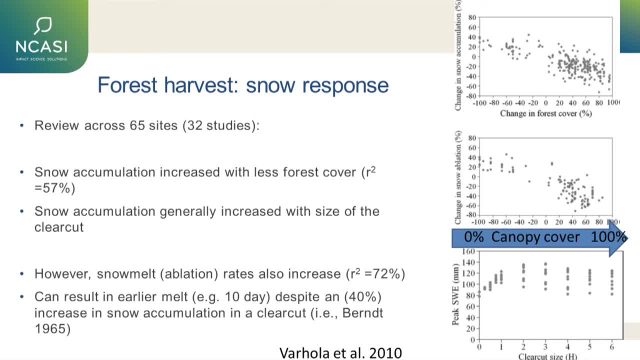 And as clear cut size increases, peak snow water equivalent increases as well. So it's basically another way to say greater snow accumulation in a clear cut area, But as we observed with the fire example also that there are increases in snow ablation or snow melt. 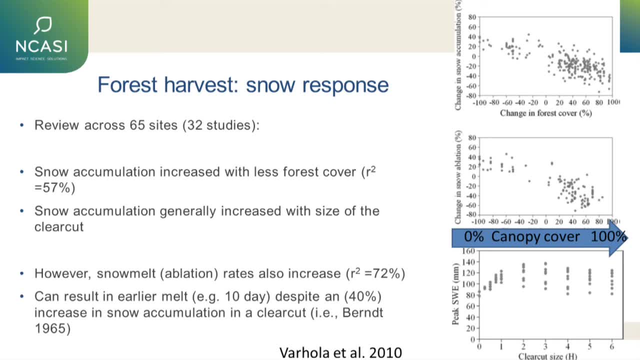 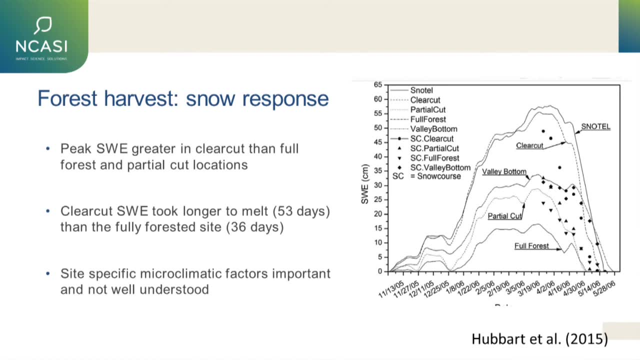 rates, And so a consequence of that is that it can actually result in earlier melt, despite having more snow available. At Micah Creek again, they have a Snowtel site there And they evaluated different snow water equivalent under a clear cut, under a partial cut. and under full forest. Here, as expected, they did observe more snow in the clear cut scenario, But they also found that it took longer to melt in the clear cut than in the fully forested area. So it took 53 days in the clear cut, related to 36 days. 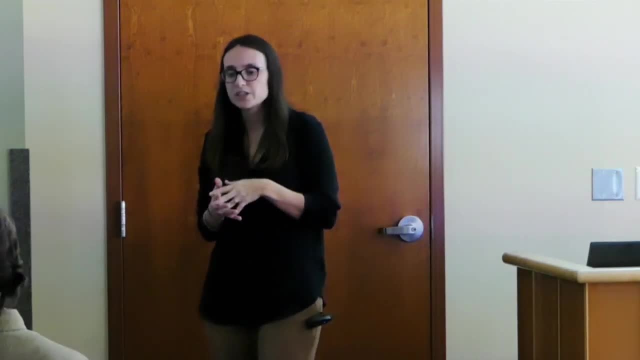 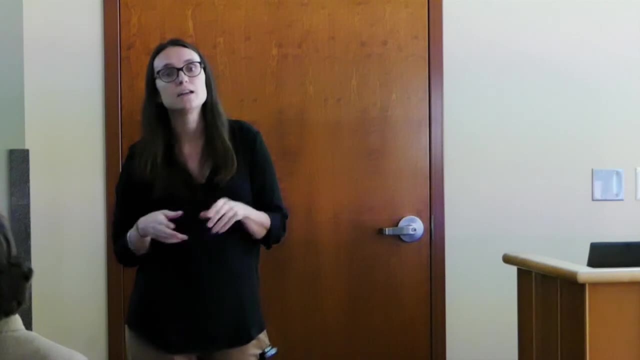 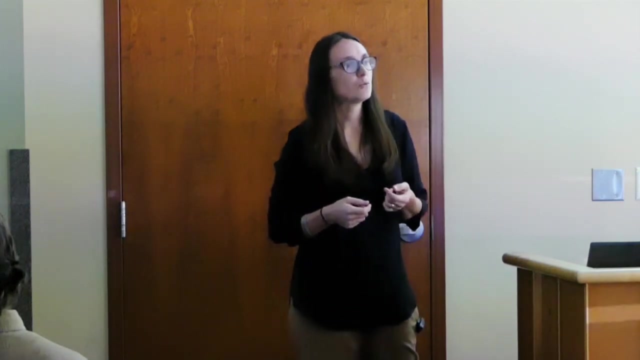 in the forested area. So this is a little bit contradictory to what the overall review says. But overall this and other studies all agree that there are a lot of site-specific microclimatic factors that are important in determining those snow melt rates which ultimately are important if we think. 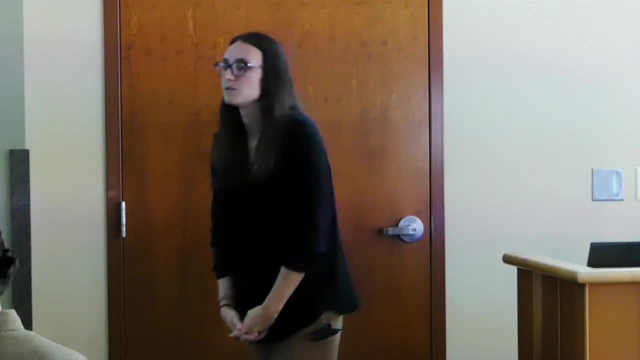 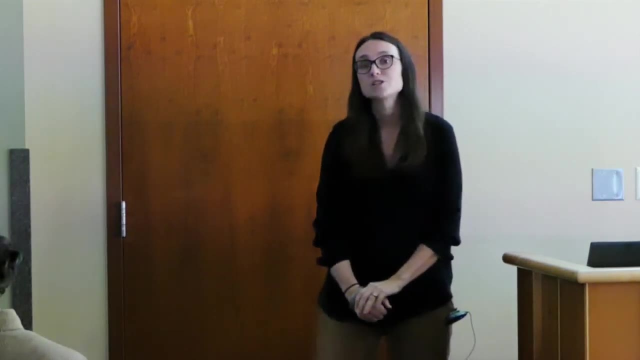 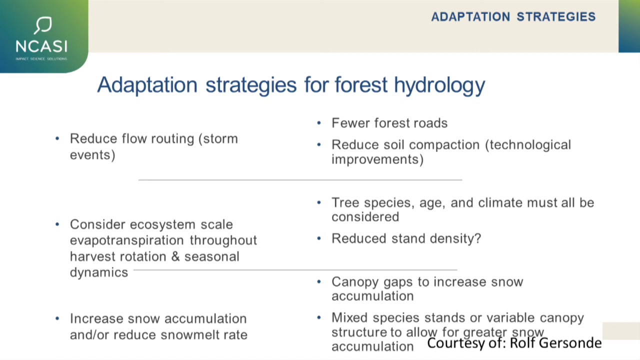 about any mitigation of strategies to increase snow, for example in the watersheds. So in terms of adaptation strategies for forest hydrology in general, if you want to reduce flow routing, so this is particularly important for storm events: obviously, fewer forest roads, reducing soil compaction. 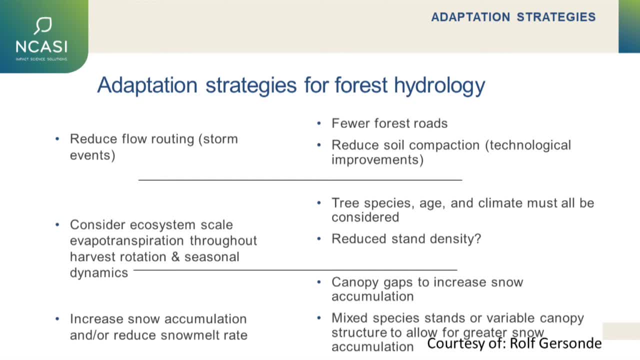 those are important strategies, But in terms of thinking about the water budget as a whole, considering ecosystem scale, evapotranspiration is important, And so that includes thinking about it throughout the entire harvest rotation and also thinking about some of those specific seasonal dynamics. 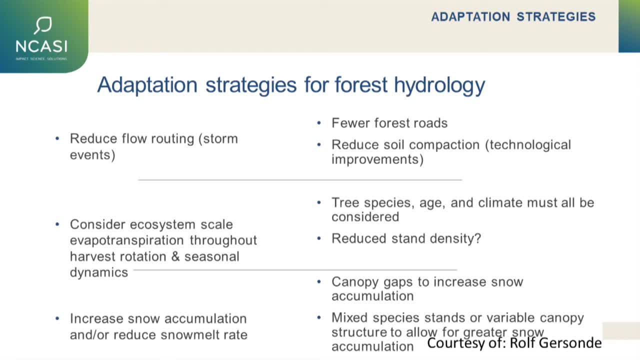 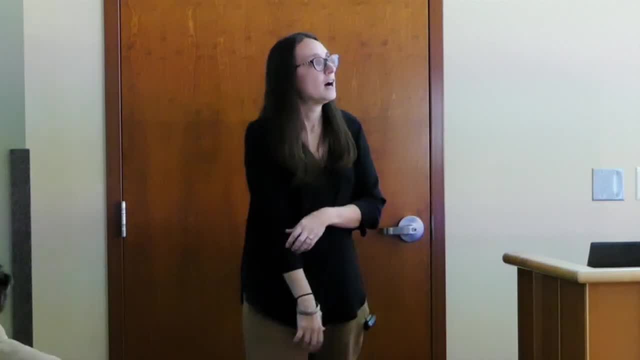 So ultimately those strategies need to consider tree species, age and climate, And there's a lot of good ideas here today already about what some of those strategies may look like. There is a question of whether or not reducing stand density will actually increase water availability. 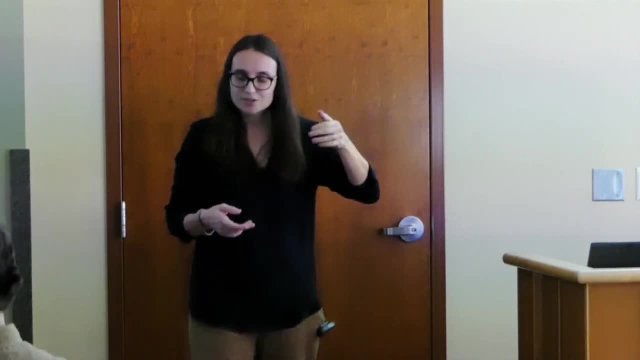 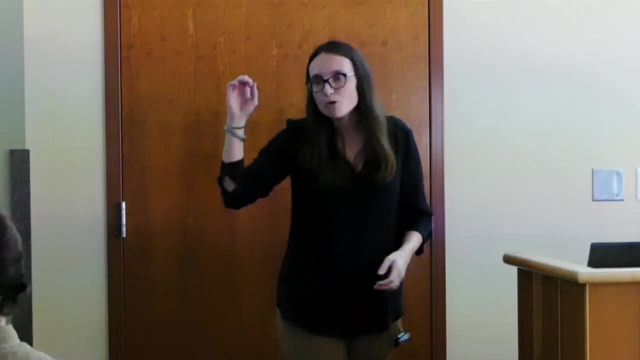 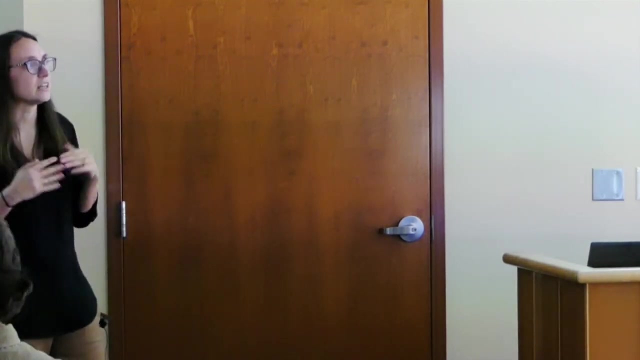 And I think using the example of the mountain pine beetle, for example. so sometimes reducing transpiration of an overstory species may not actually reduce evapotranspiration at the ecosystem level, And I think this is still a question where we need more research. 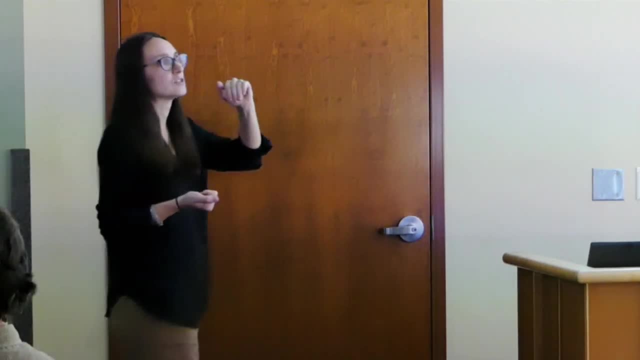 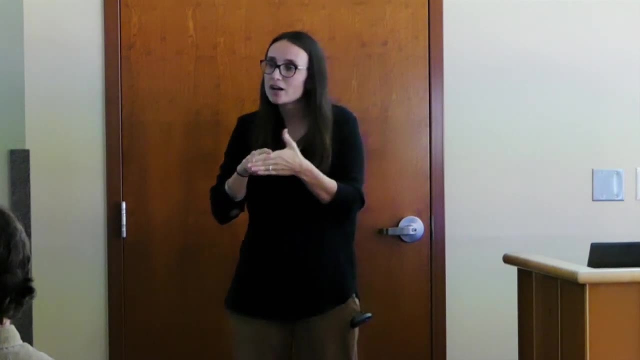 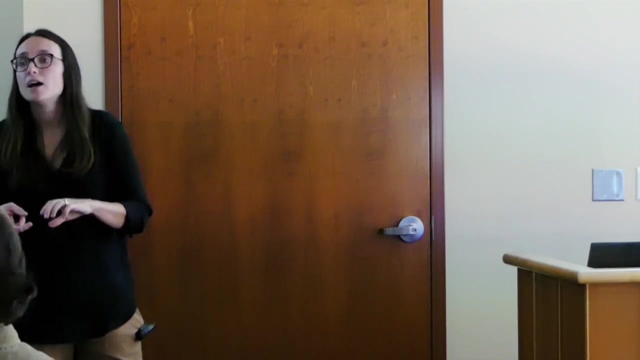 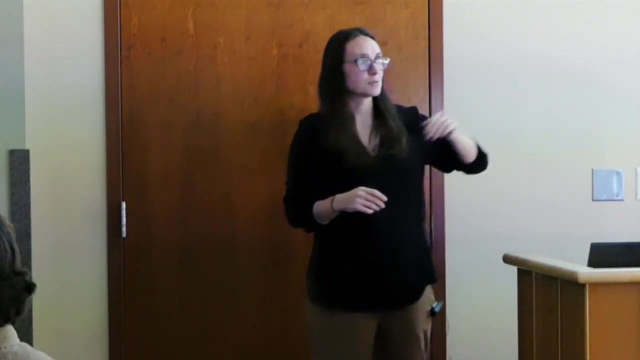 And so, even if transpiration is reduced in the predominant species, there's a question of how long it will take for the ecosystem to recover, either through understory vegetation, transpiration processes or also evaporation processes within that system. And then, finally, as I just mentioned,